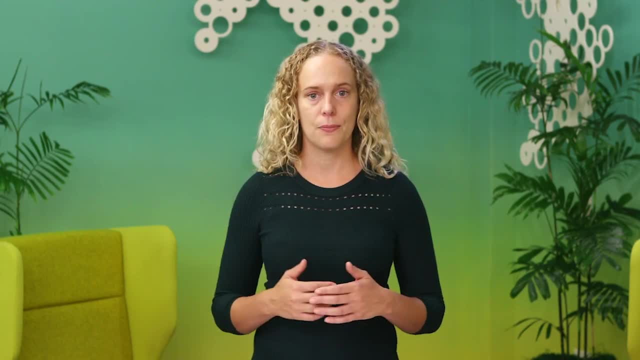 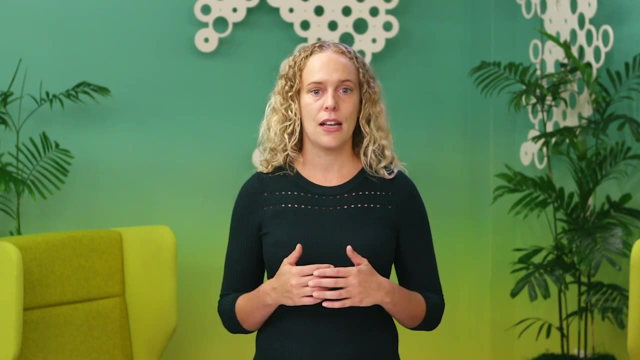 management, you'll think about them as hypothetical. In other words, these aren't events that will definitely happen, but because there's a possibility that they could happen, it's your responsibility as the project manager to identify and plan for those risks. Next, 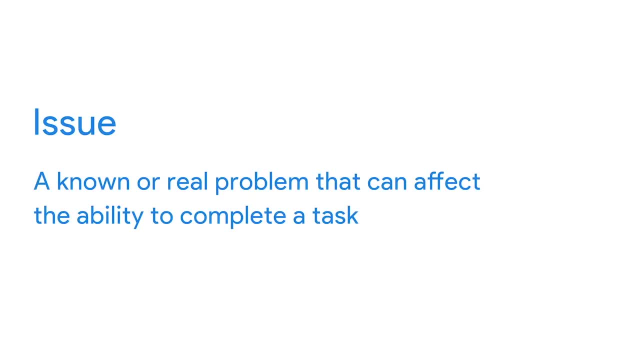 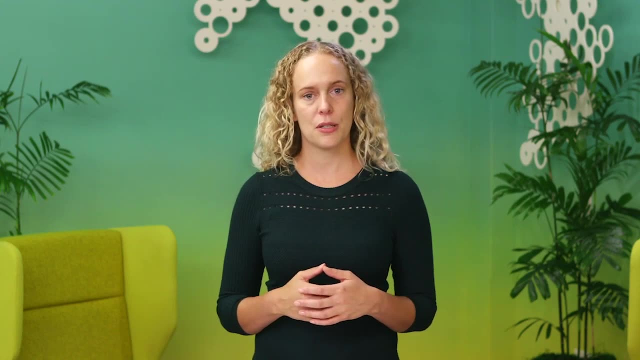 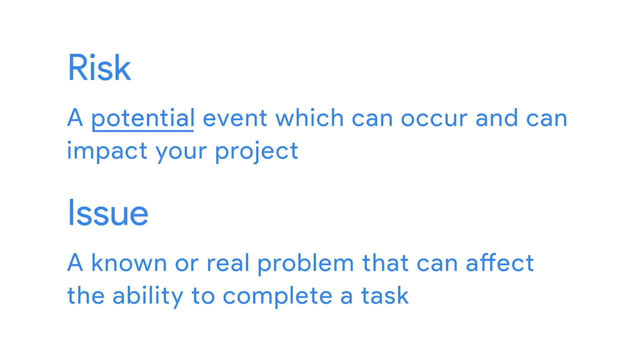 let's discuss issues. An issue is a known or real problem that can affect the ability to complete a task. So what's the difference between a risk and an issue? Think of it like this: A risk is an event that could potentially happen. If the event actually happens, then the risk becomes an issue. 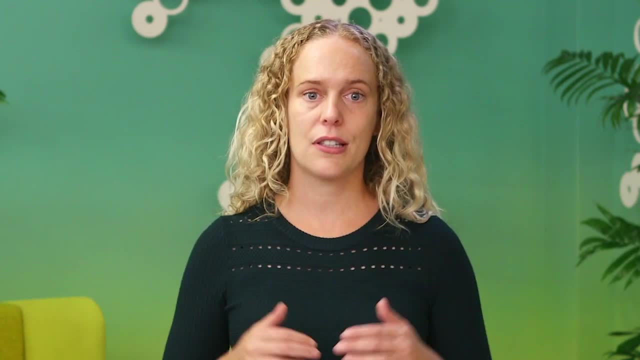 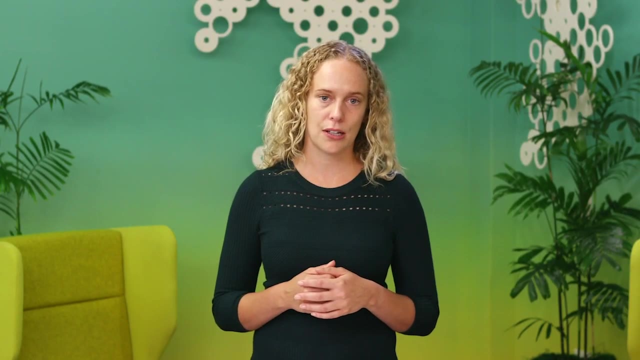 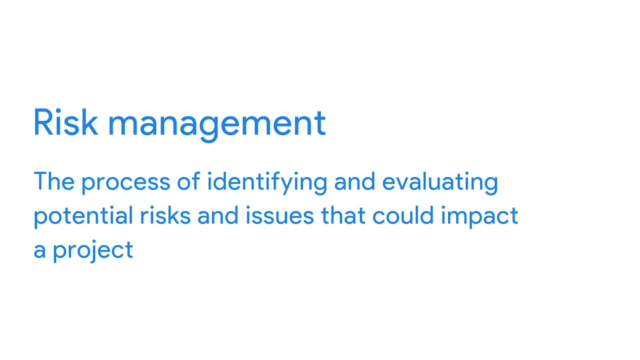 In other words, risks are the big what-ifs and issues are things that currently impact a project. It is clear that risks and issues can pose a threat to your project. How you manage those risks is known as risk management. Risk management is the process of identifying and evaluating. 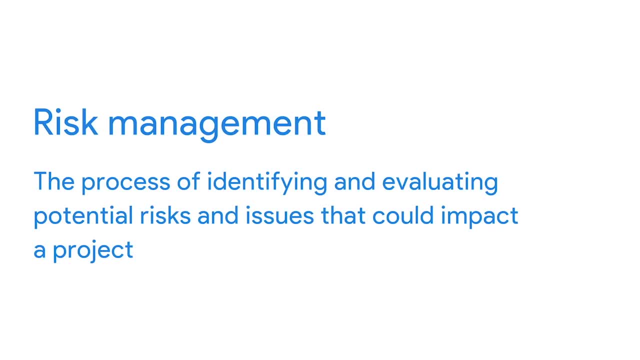 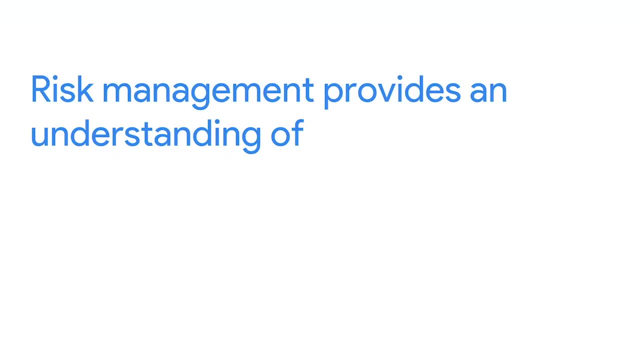 potential risks and issues that could impact a project. It's not a one-time exercise. It's something that you'll need to do regularly to address potential risks. Risk management is a crucial part of the planning process. by giving you an understanding of what could go wrong with your project, It also tells you who you need to consult about the risk. 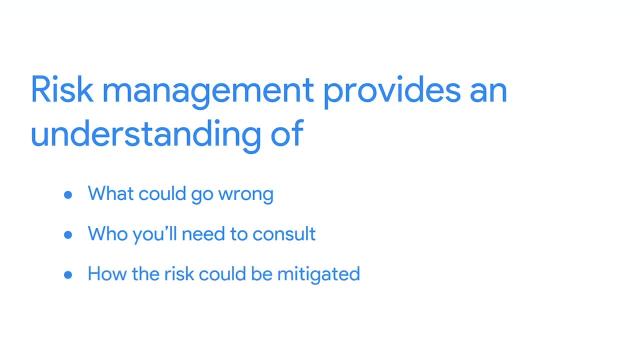 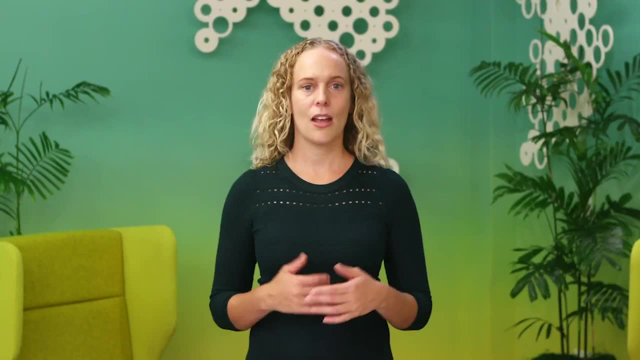 It helps you determine how the potential risk could be mitigated. This way, if or when something goes wrong, you'll have a plan prepared and ready to go. Part of being proactive and planning ahead is identifying potential risks and how to solve for them. 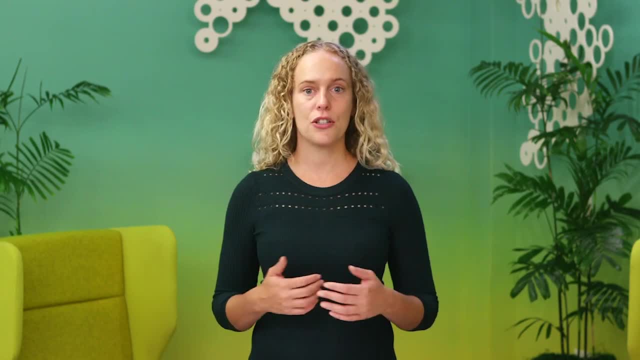 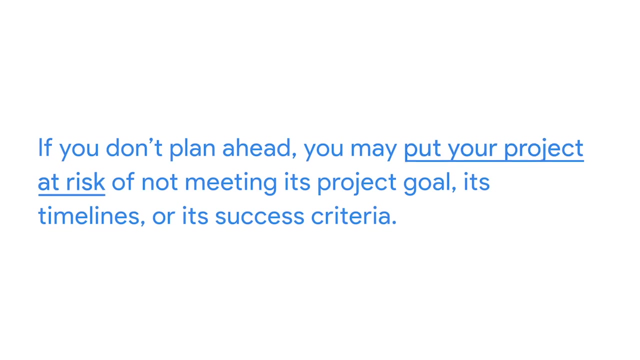 This way, you'll set up your project with better chances for success. Failing to engage in meaningful risk management can have a few big consequences for your project. First, if you don't plan ahead, you may put your project at risk of not meeting its project goal. 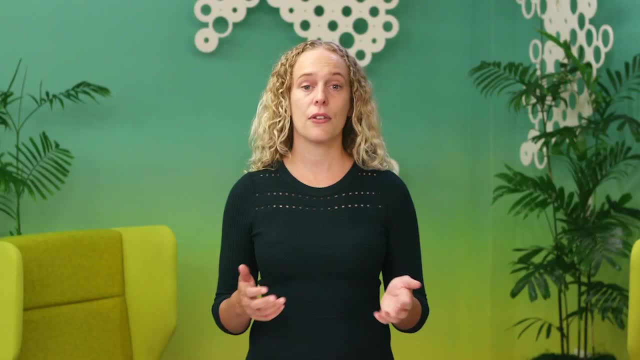 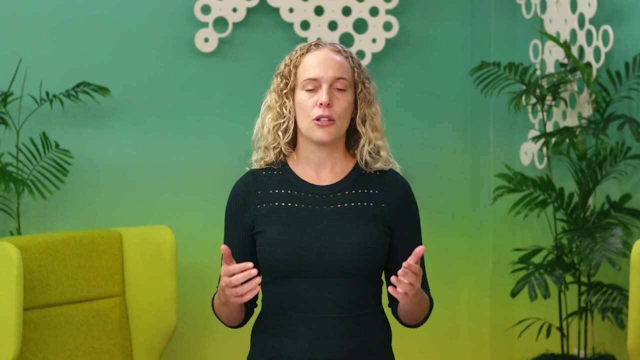 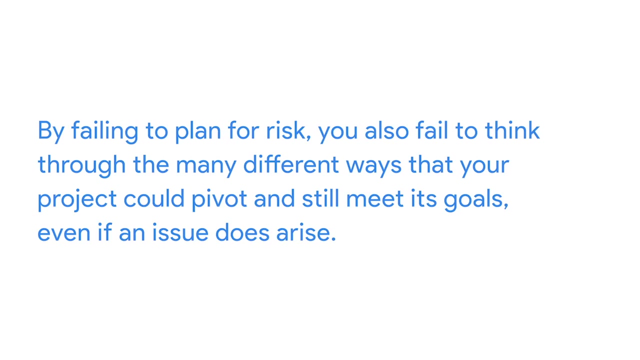 its timelines or its success criteria. For example, if your goal is to publish a research report and your research analyst quits halfway through the project, you'll likely miss the deadline if you don't have a backup plan ready to go. Additionally, by failing to plan for risks, you also fail to 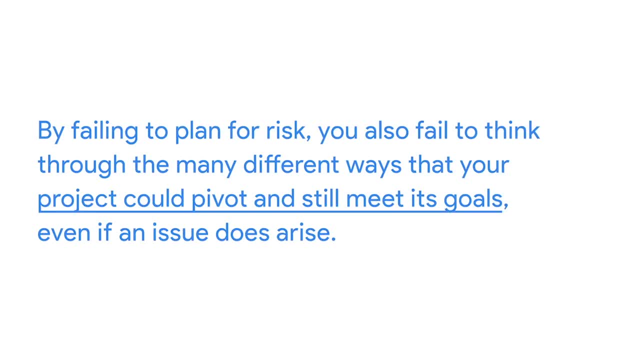 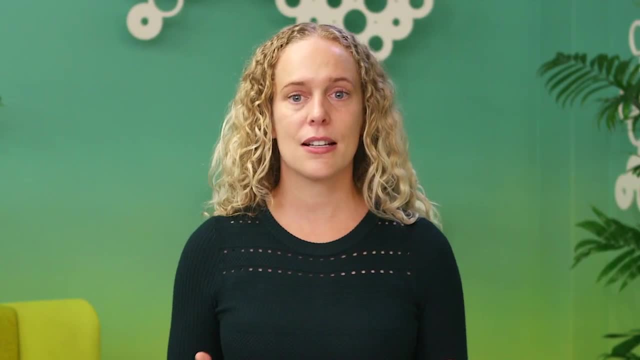 think through the many different ways that your project could pivot and still meet its goals, even if an issue does arise. There often isn't just one way to meet your project goals, and success can come in many forms. Risk management helps you determine how flexible. 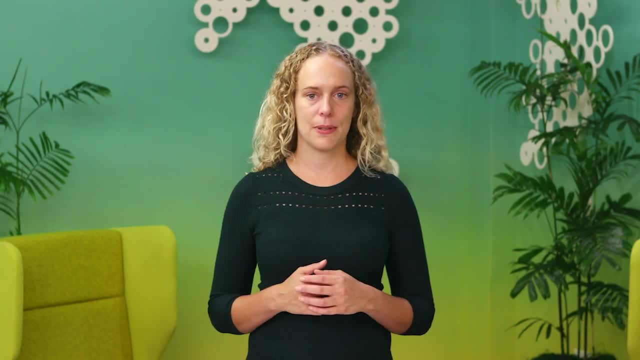 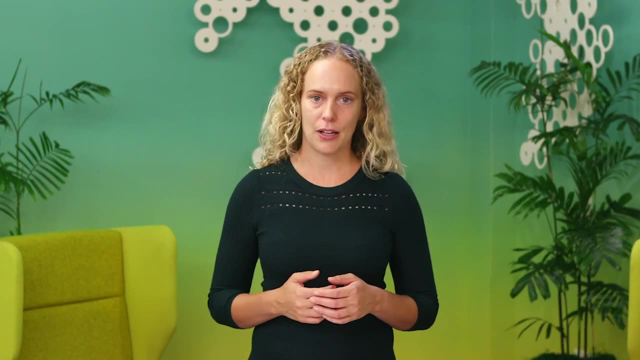 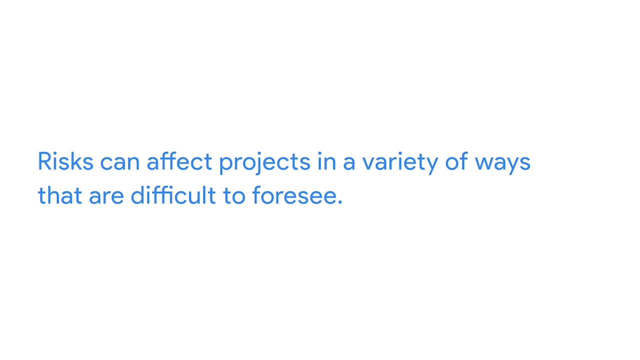 or rigid your plan is and then make necessary adjustments. For example, if your project requires a large product shipment, having a backup supplier ready means you could quickly pivot if our main supplier is unable to fulfill your order. Finally, risks can affect projects in a variety of ways that 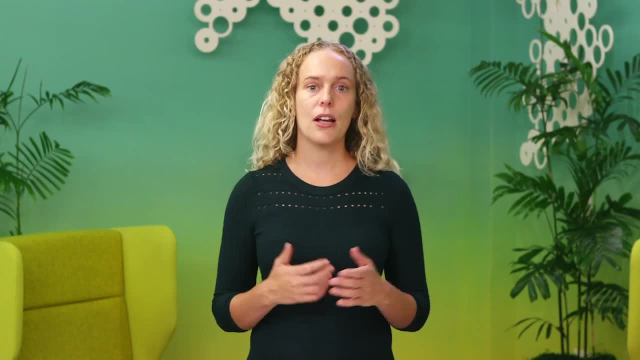 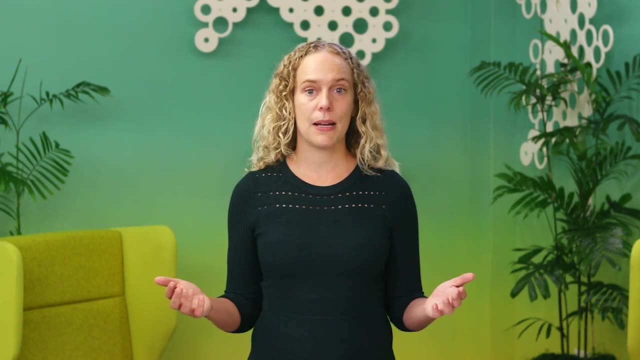 are difficult to foresee. For example, a supplier you've hired may not have adequate stock to cover your purchasing needs, or the budget for your project could be cut unexpectedly. The risk management process helps reduce the impact of unexpected events, freeing up resources. 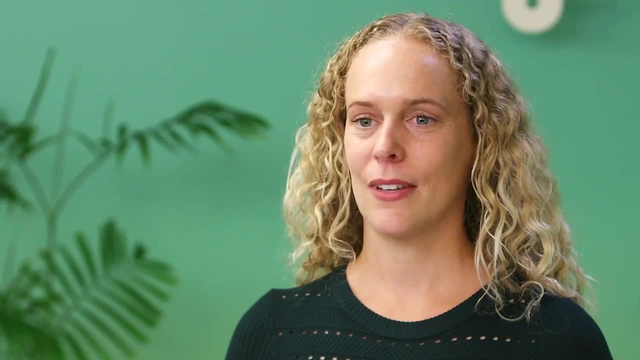 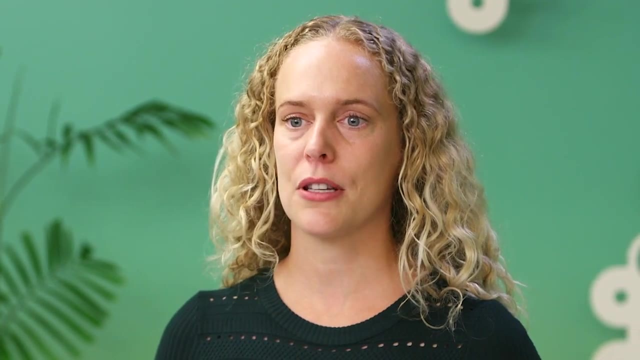 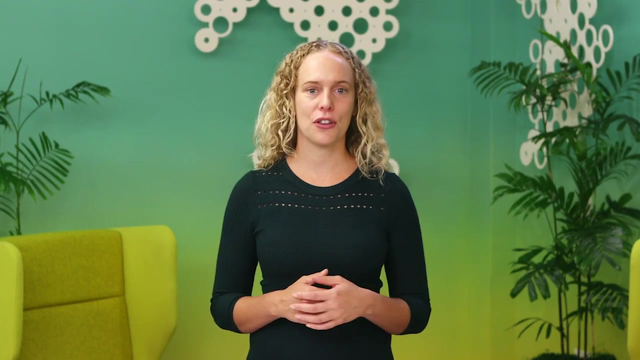 to focus on activities that benefit the project. Let's imagine risk management in the context of PlantPals at OfficeGreen, which is a new service that will provide customers with small, low maintenance desk plants. One potential project risk is the possibility that the webpage for the 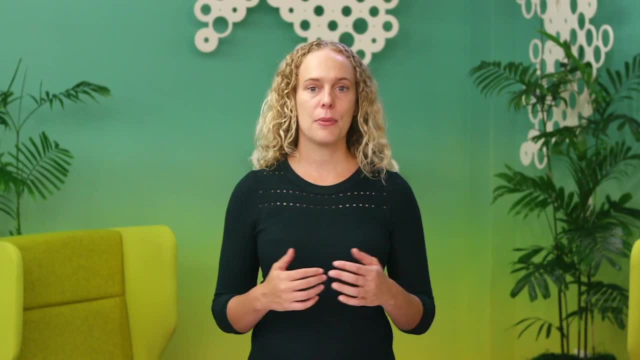 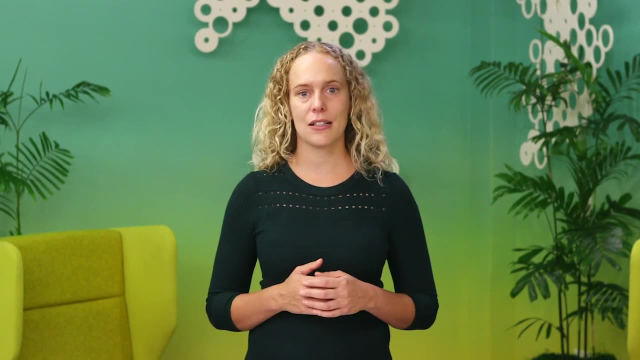 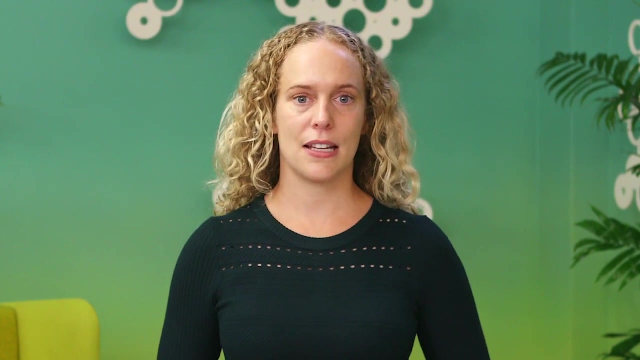 new service won't be live in time for the launch. Another potential risk could be a fulfillment shortage. What would you do if the plant supplier runs low on the cacti and ferns that you need To prepare for these potential risks. you will need to think about ways to mitigate these issues. 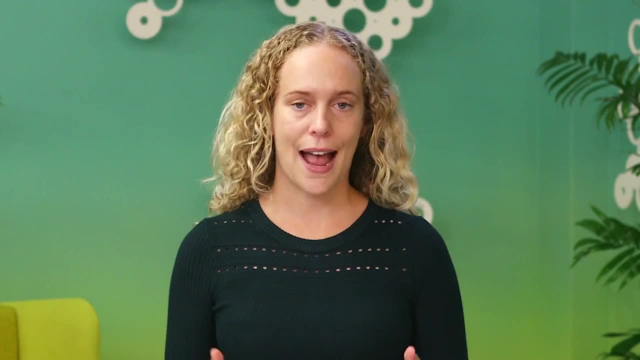 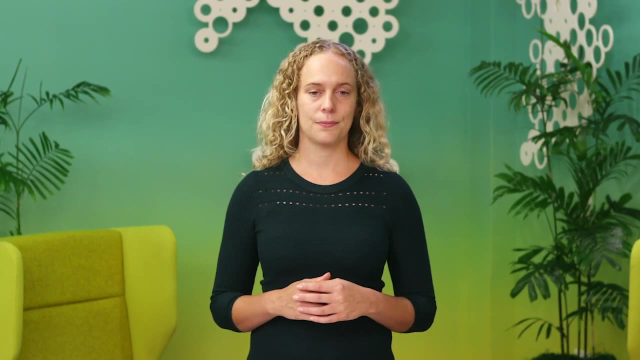 before they happen, or how you will address these issues if they actually occur. Hopefully, these things won't be a problem, but if they are, you'll be prepared. I also want to stress that issues will come up throughout the project. you did not or could not. 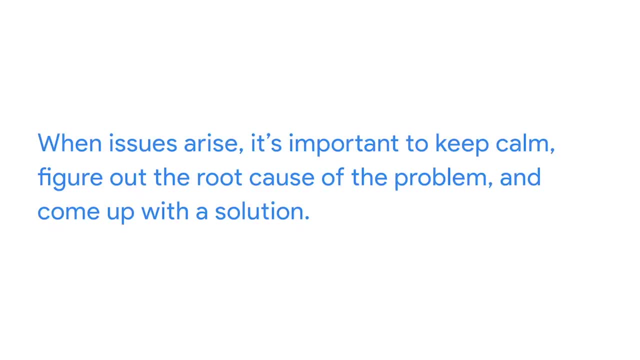 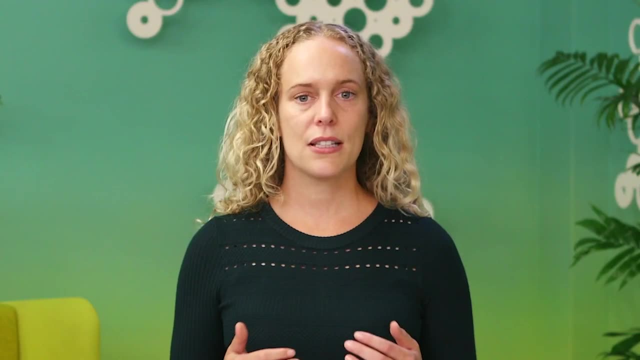 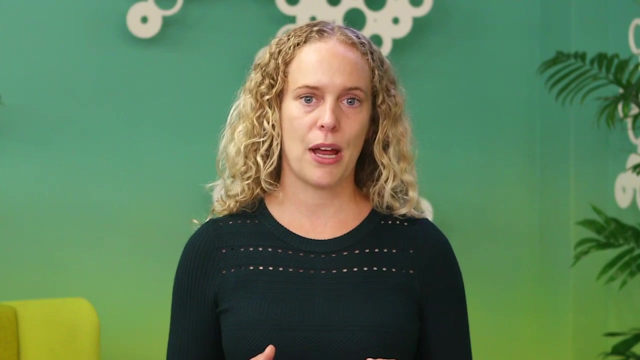 have planned for, And that's okay. When these moments arise, it is important to keep calm, figure out the root of the problem and come up with a solution. Risk management is a really important topic for project managers to understand. Identifying risks and issues prepares you for the unknown. 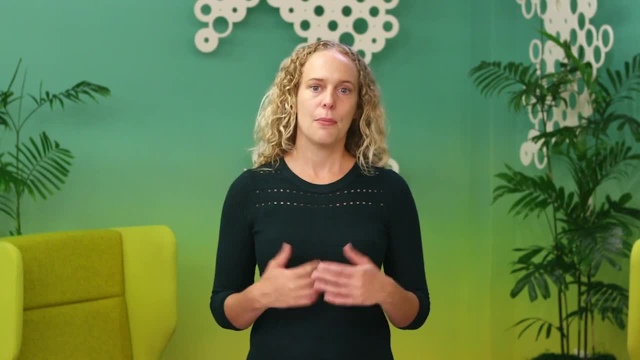 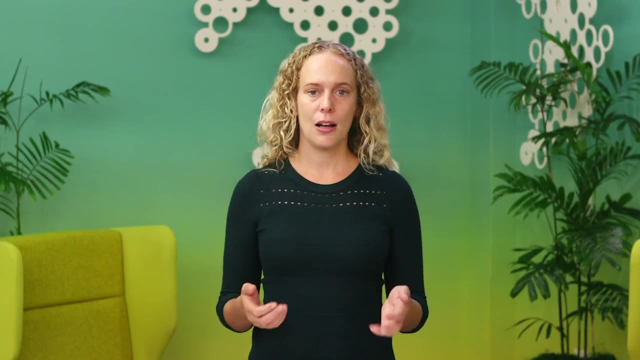 It also positively impacts you as the project manager, because you'll feel more prepared, less stressed and more confident in your approach if an issue does occur. Up next we will discuss ways that you can identify risks. I'll meet you there. 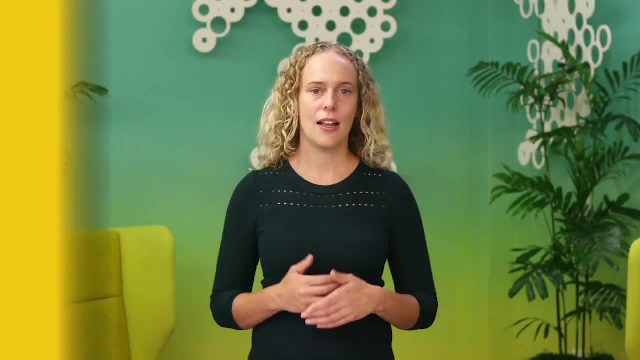 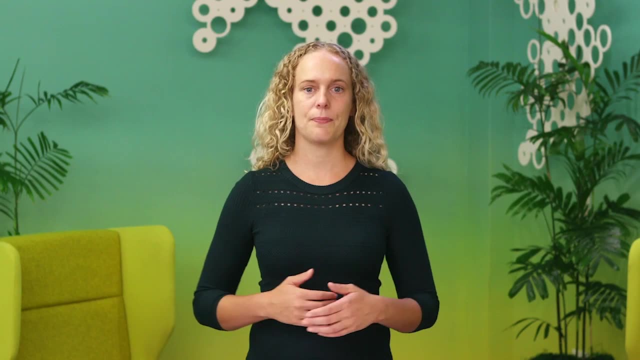 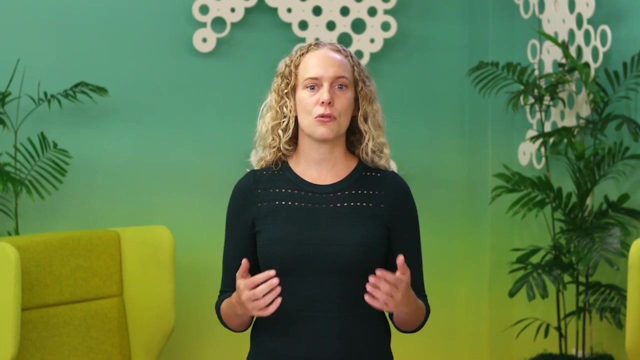 Let's discuss tools and techniques you can use to identify risks, including brainstorming and risk assessment. Brainstorming is one of the most effective techniques for identifying risks with a team because it allows groups to spontaneously share ideas without judgment. As a project manager, 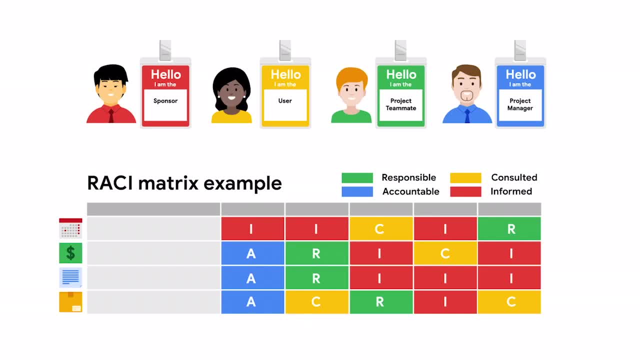 you will be responsible for bringing a group of people together to imagine potential risks. Have your RACI chart at the ready to refer to when you decide who to invite to this meeting. Speaking from experience, the best team for this task is a diverse one which includes individuals. 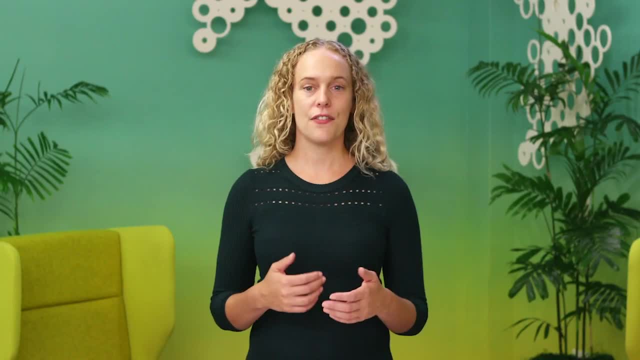 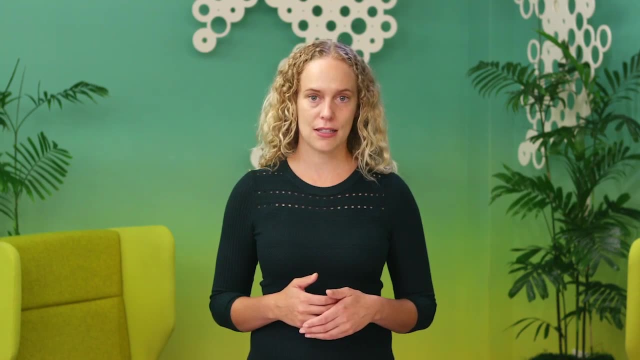 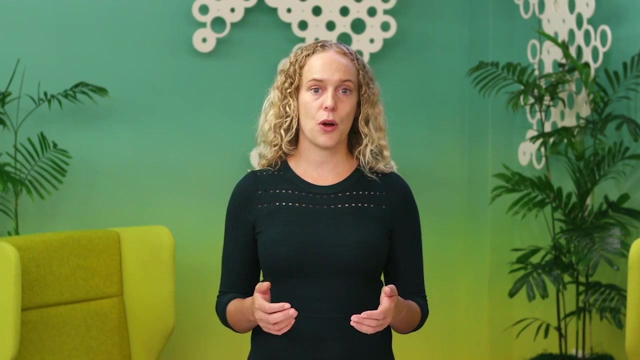 from various roles, backgrounds and experiences. Diverse teams bring different perspectives, experiences and skill sets, and this may help you to identify risks that you may not have thought of on your own. For example, one member of your team might have experienced working. 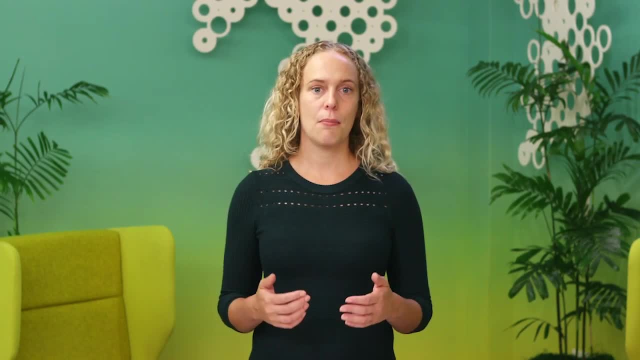 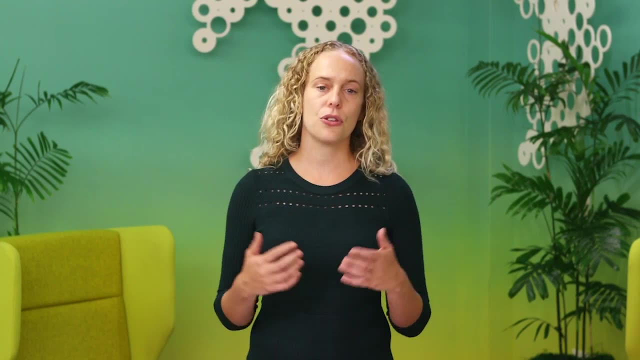 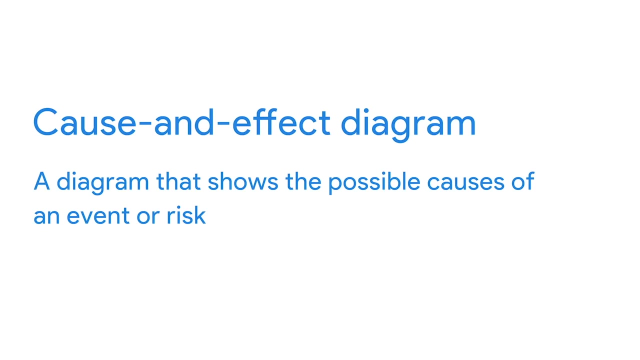 on multiple projects, while another newer team member might bring a fresh perspective from their previous experience on other teams. A great tool that you can use during brainstorming is called a cause and effect diagram, also sometimes known as a fishbone diagram. Cause and effect diagrams show. 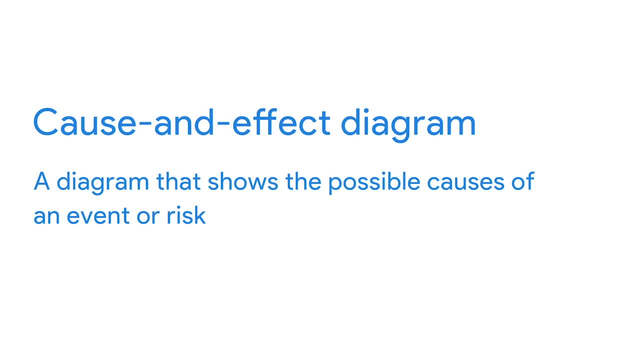 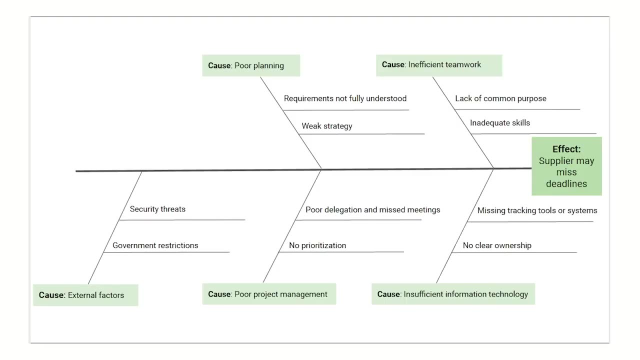 the possible causes of an event or risk and are very useful at risk management. For example, in the diagram seen here, the effect listed is a fire missing its deadlines. This is a risk to your project. On the left, you'll brainstorm potential. 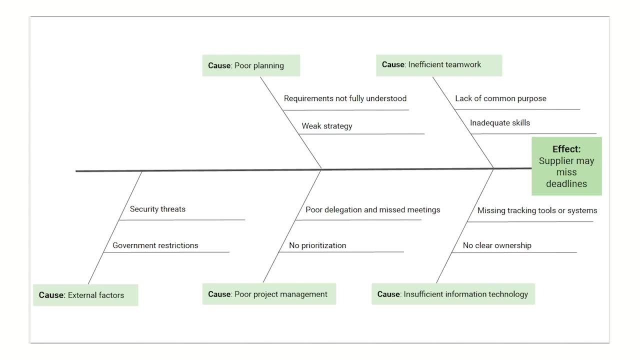 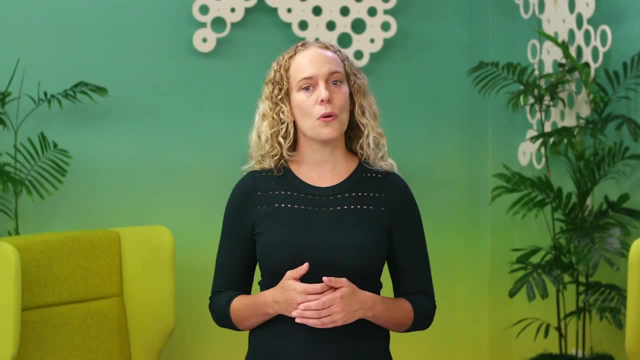 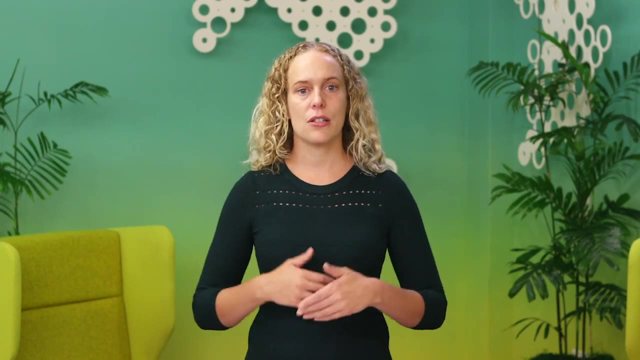 causes that would lead to the effect, like poor delegation or a lack of tracking tools. In other words, cause and effect diagrams can help identify all the ways that things could go wrong by identifying a potential risk, known as the effect, and working backwards to 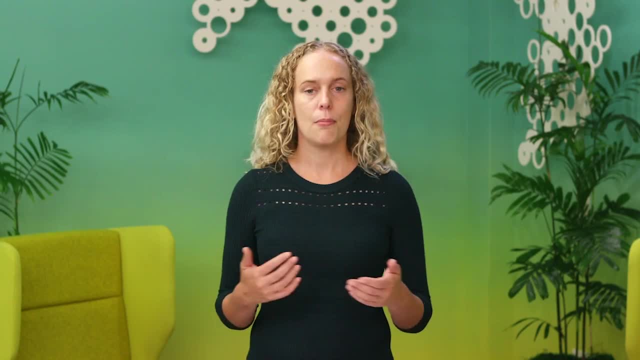 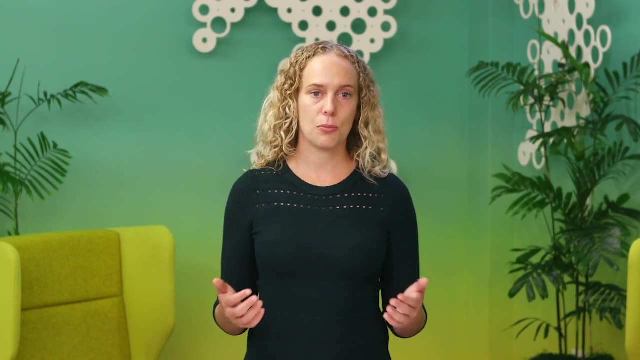 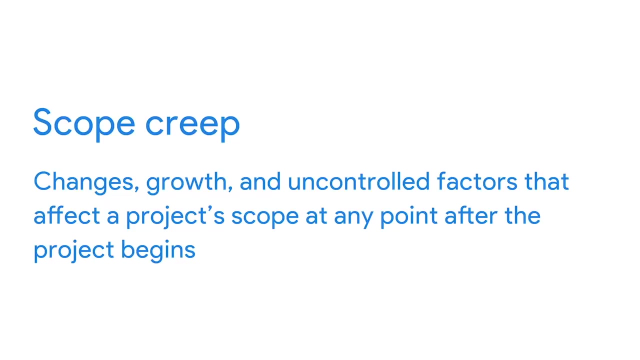 consider the potential causes of that risk. By categorizing and breaking them down into further causes, you are able to identify areas that could lead to a potential problem, like exceeding your budget or allowing scope creep to impact your timeline. As a reminder, scope creep refers to changes, growth and uncontrolled factors that affect a 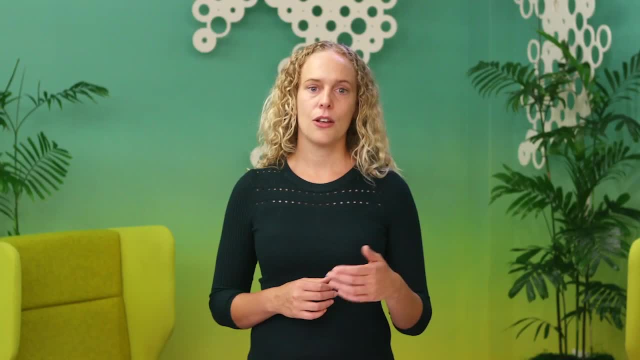 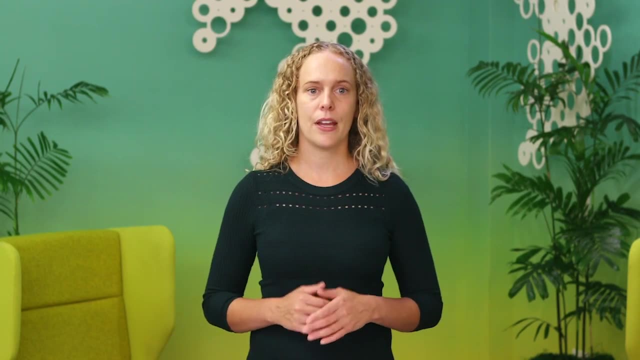 project's scope at any point after the project begins. During these brainstorming sessions, you might find that your list of potential risks is quite long, and that's ok, It is a reality. You, your team, cannot account for every single problem that can occur during. 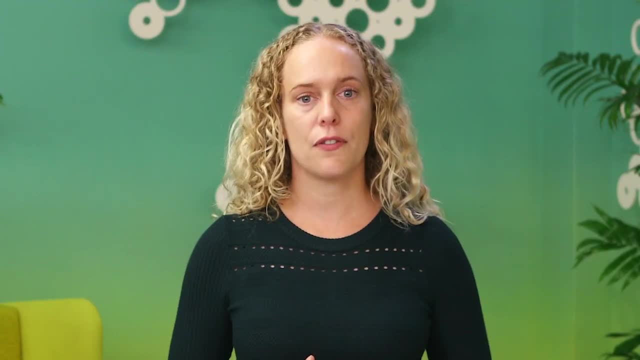 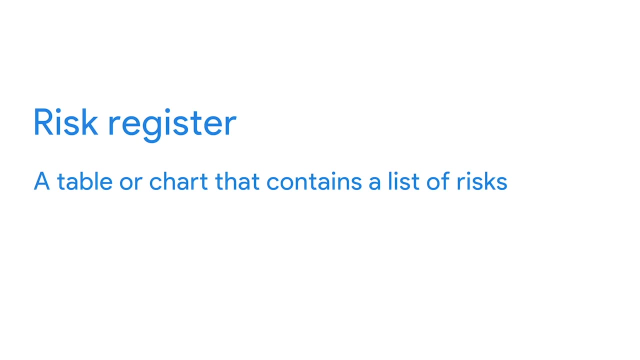 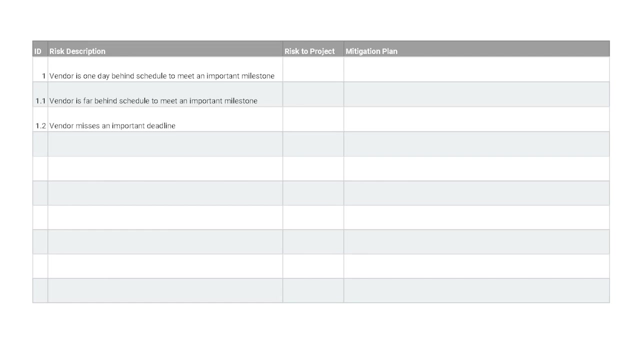 your project. So how do you decide which risks to focus on? List the outcomes from the brainstorm in a risk register. A risk register is a table or chart that contains your list of risks. Next you'll adopt a risk assessment technique. Risk assessment is the stage of risk management where qualities of a risk are. 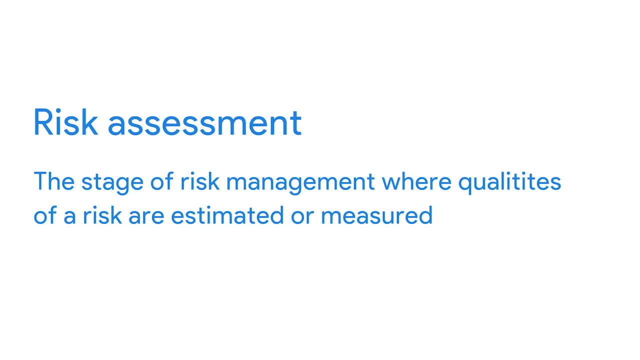 estimated or measured By qualities. we're mainly referring to how likely the risk is to occur and its potential impact on a project. We'll come back to this point in a moment. There are a few ways to assess risks, but one we'll focus on is 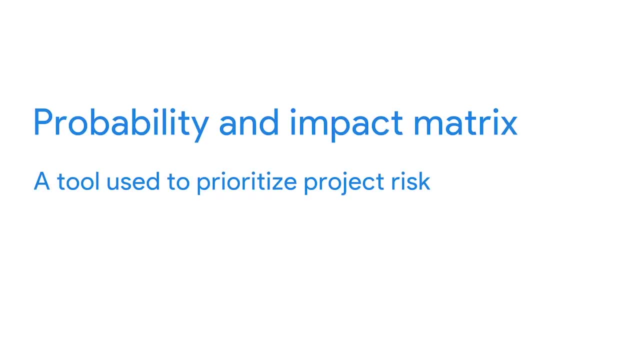 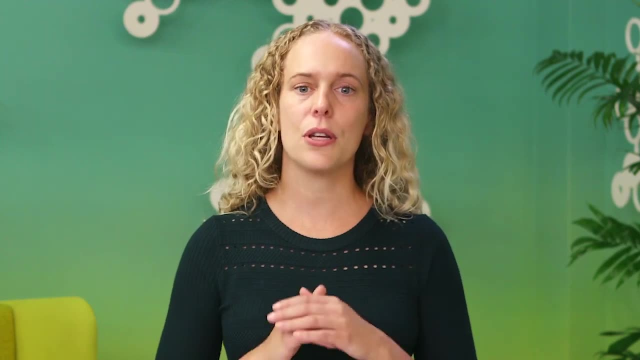 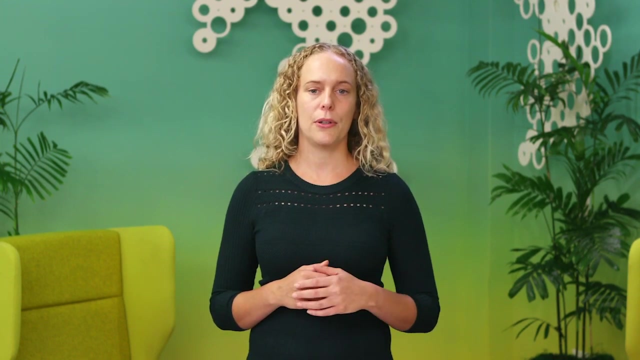 creating a probability and impact matrix. A probability and impact matrix is a tool used to prioritize project risks. I personally love this technique and use it all the time in my role at Google. Earlier, I mentioned that you'll need to assess the likelihood that a risk will. 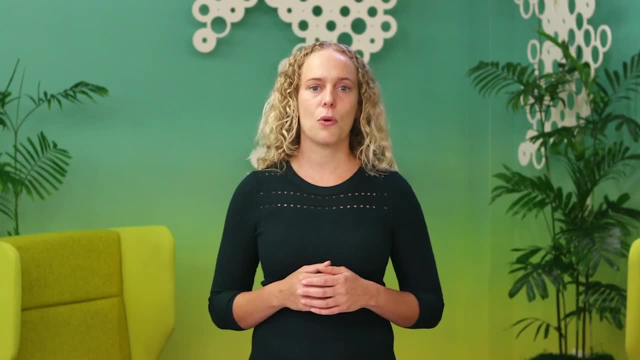 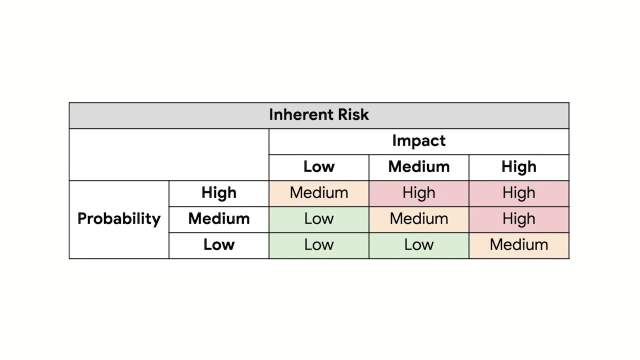 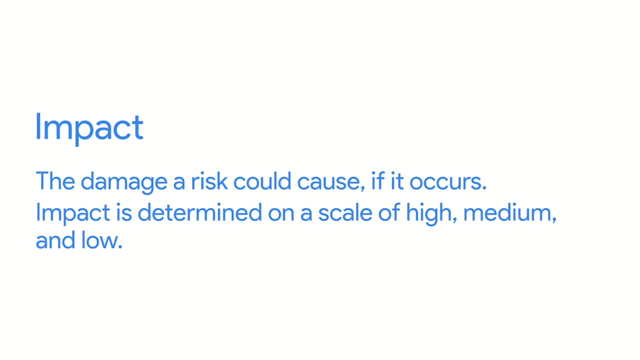 happen and its potential impact. This matrix will help you do just that. To create a probability and impact matrix, you'll need to think about the level of impact. Impact refers to the damage a risk could cause if it occurs. Impact is also determined on a scale of high, medium and low. High means that if the 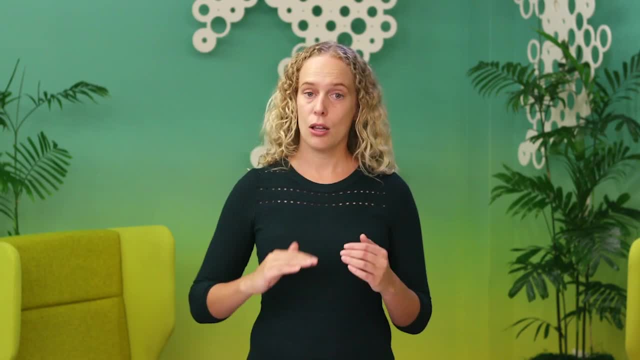 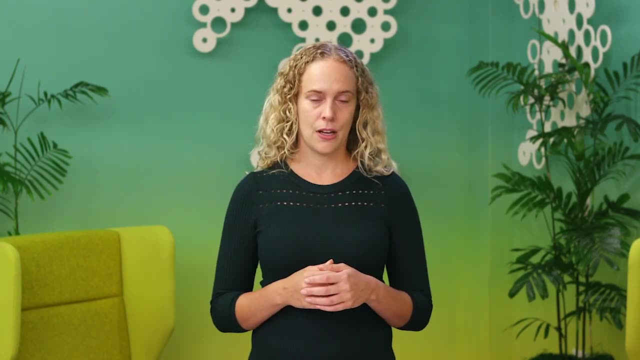 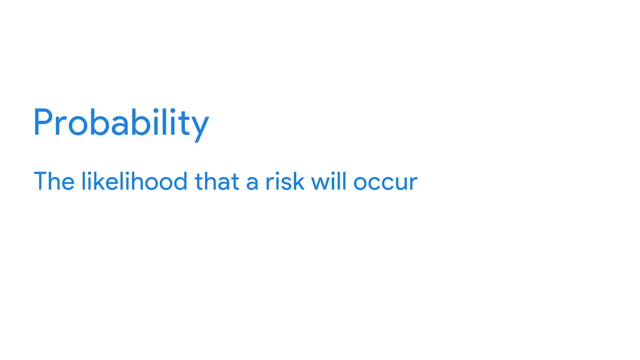 risk occurs, it will substantially alter the project. Low means if the risk occurs, it will have a slight impact, but it's not likely to derail the project. You'll also need to think about probability. Probability is the likelihood that a risk will occur. We also determine probability on a scale of. 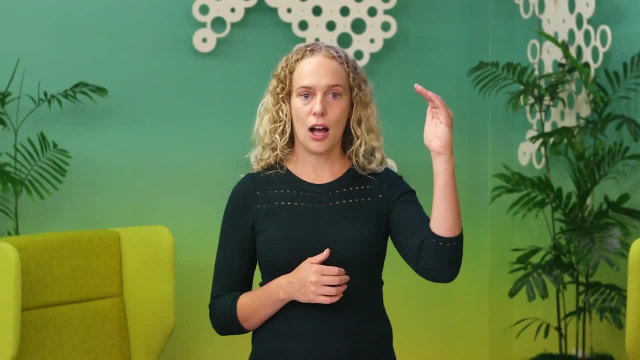 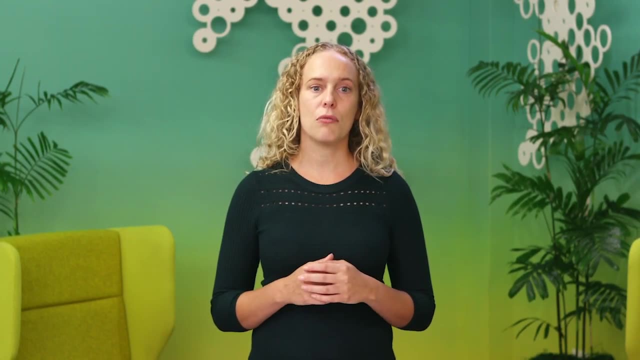 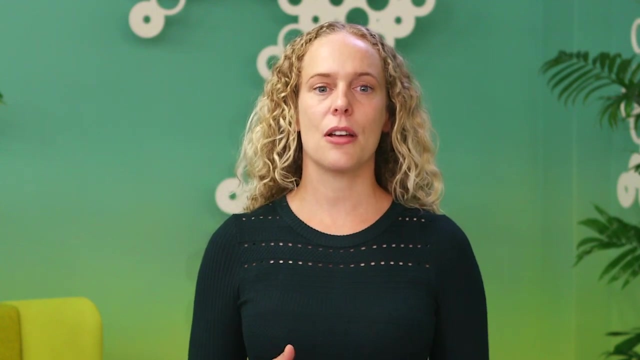 high, medium and low In this case. high probability means there's a high likelihood of this happening. Low probability means you've identified a risk that could happen, but it isn't likely that the risk will occur. The risk occur. These two considerations come together to determine the inherent risk rating. Inherent risk. 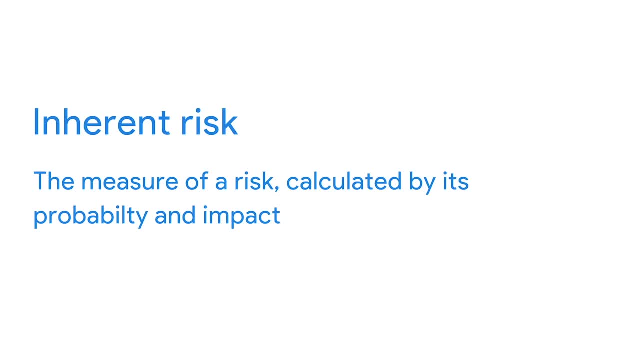 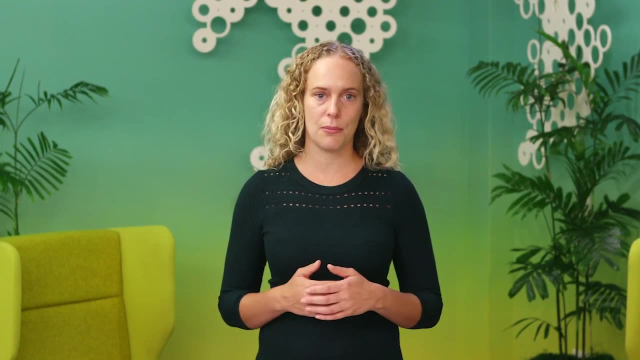 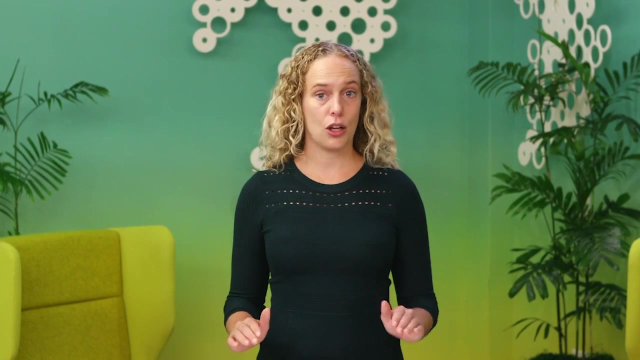 is the measure of a risk, calculated by its probability and impact. Measuring the inherent risk gives us a method for understanding a risk. Inherent risk is also determined on a high, medium and low scale. So basically, if a risk has a low impact and a low probability. 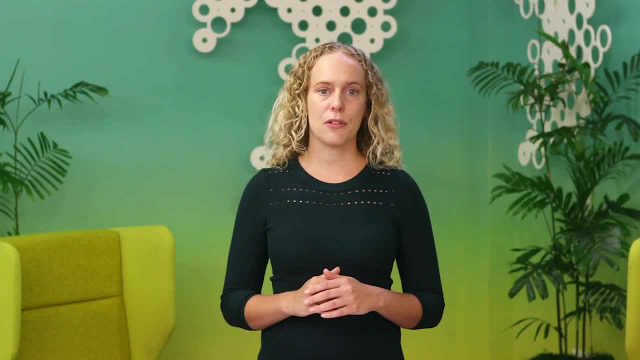 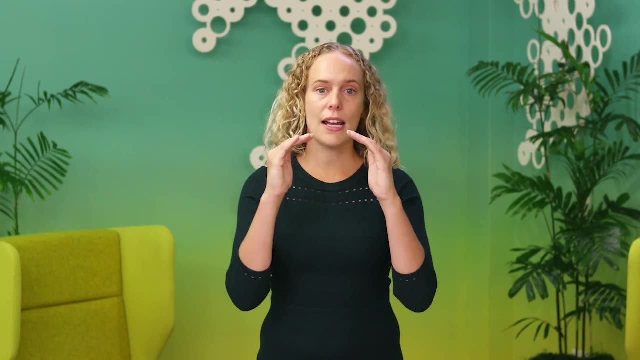 it has a low inherent risk rating. These are the types of risks you don't need to worry too much about, But if a risk has a high impact and a high probability, then it carries a high inherent risk rating. Medium to high risks are the risks you should focus on and create detailed mitigation. 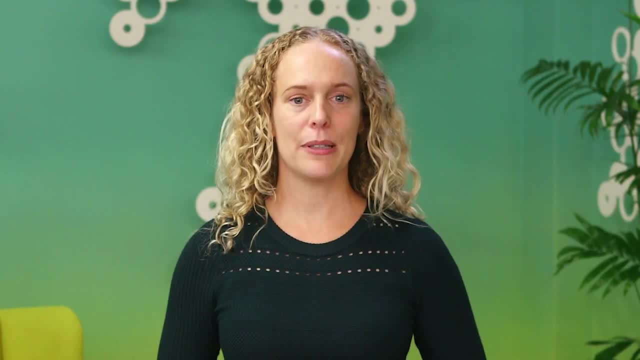 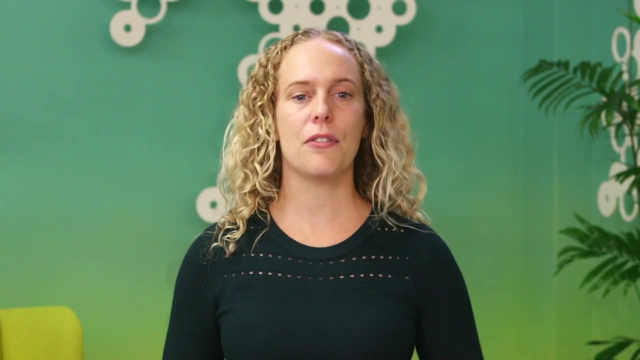 plans for When you're creating a probability and impact matrix. it's important to ensure you create a matrix that meets accessibility guidelines and has information and formatting that everyone can easily use. If you are using a high risk medium, you can use the probability. 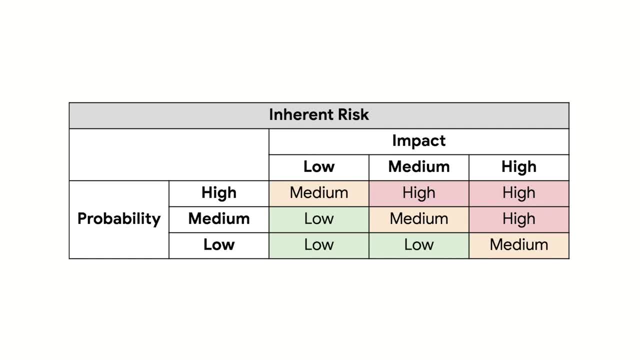 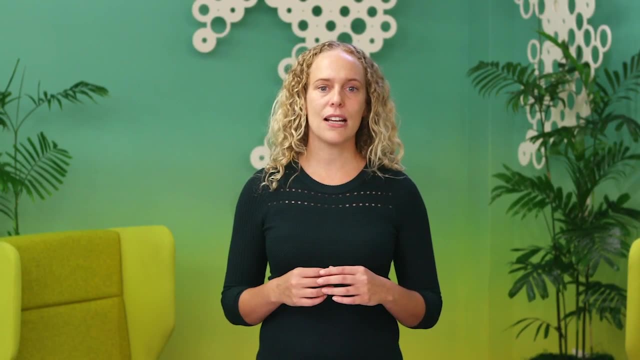 and quickly understand. One way to do this is to use both color and distinct shapes or text to communicate levels of risk. You can learn more about accessibility communication by visiting course resources. The way you view and manage each risk will be determined based on your organization's. 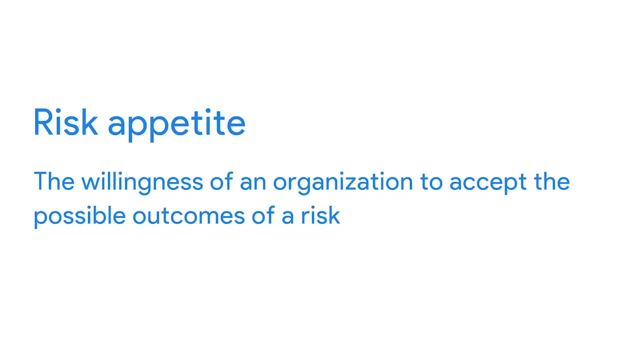 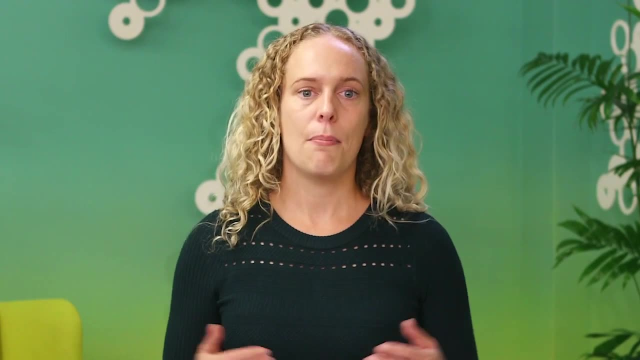 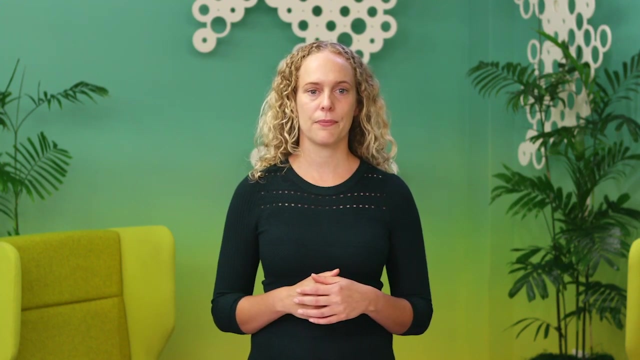 risk appetite, which refers to the willingness of an organization to accept the possible outcomes of a risk. You, your team and your stakeholders may have different appetites for each risk. We'll discuss how risk appetite plays into risk mitigation in just a bit. 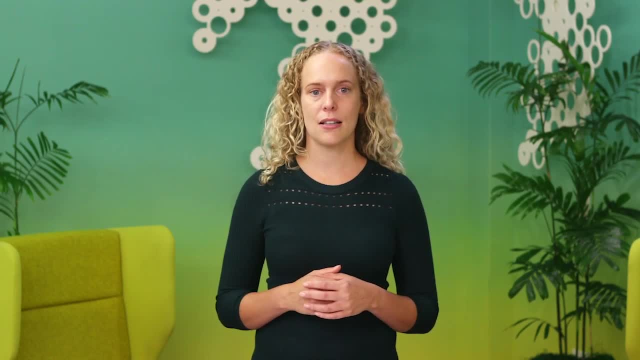 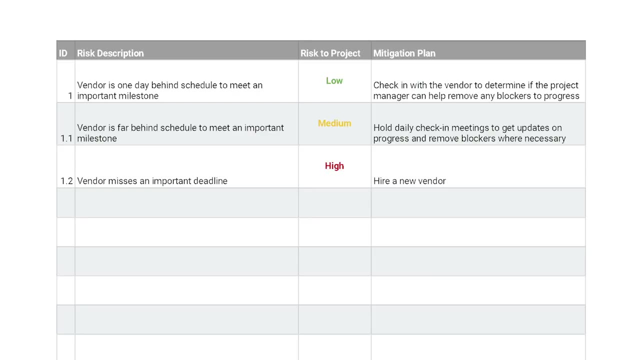 Certain low-level risks that could result in minor setbacks are much more tolerable than high-level risks that have the potential to completely derail your project. Once you've completed your risk assessment, you'll update the risk register to include high, medium and low ratings for some examples of risks. 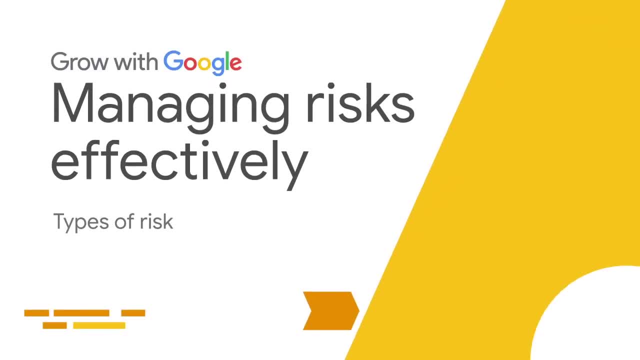 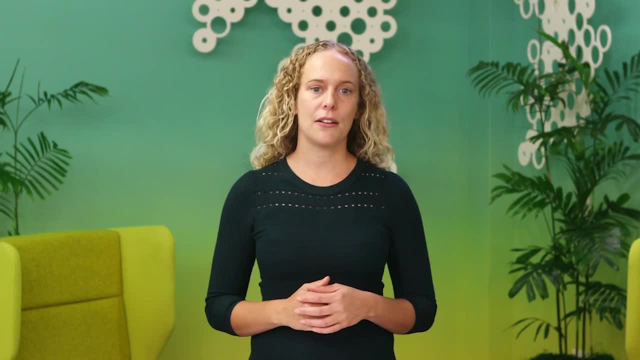 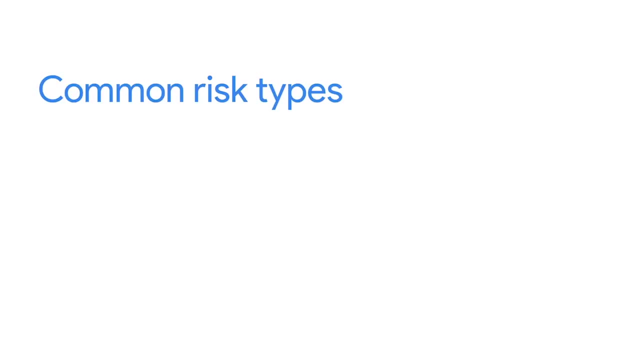 that you've identified for this project. Let's discuss some common types of risks that you might plan for while managing a project. Though there are many different types of risks that could impact your project, the big ones that you want to be aware of are time risks, budget risks. 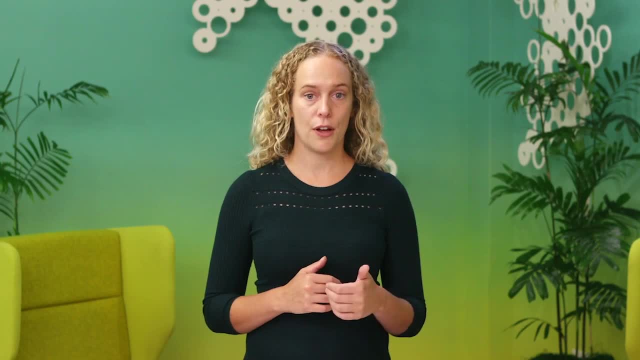 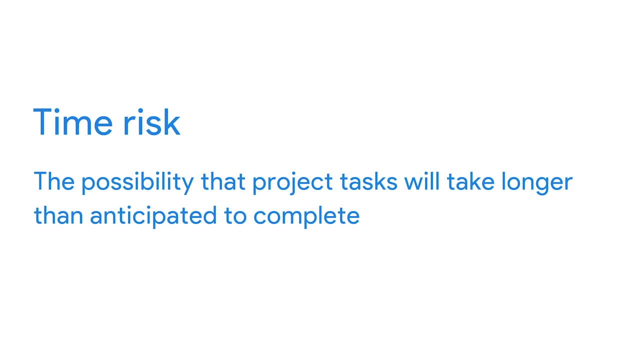 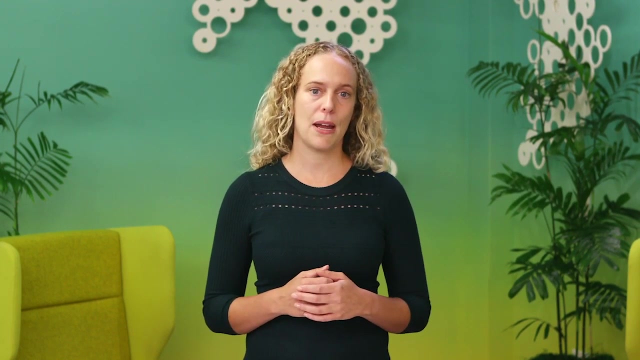 and scope risks. Let's break those down. First, we have time risks. Time risk refers to the possibility that project tasks will take longer than anticipated to complete. You'll need to be aware of time risks because time is money. Poor time management may deplete your budget. 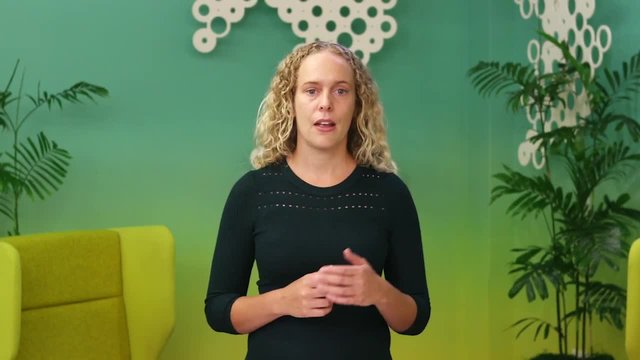 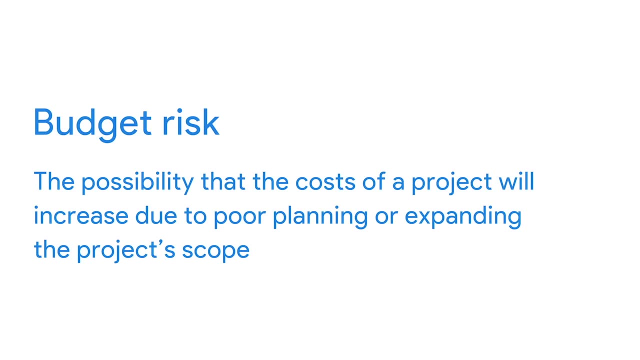 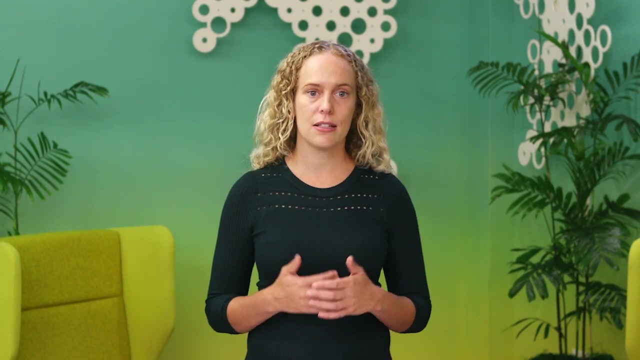 and upset your stakeholders by causing delays. Next, we have budget risk. Budget risk refers to the possibility that the cost of a project will increase due to poor planning or expanding the project's scope. You need to be aware of budget risk, since budgeting provides the basis. for project costs control, For example. if you overspend, you might not be able to pay your suppliers. This could also result in some reputational damage for the company. Then we have scope risk. Scope risk refers to the possibility that a project won't produce the results outlined. 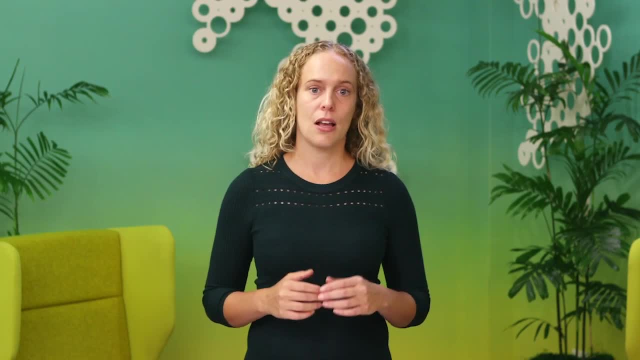 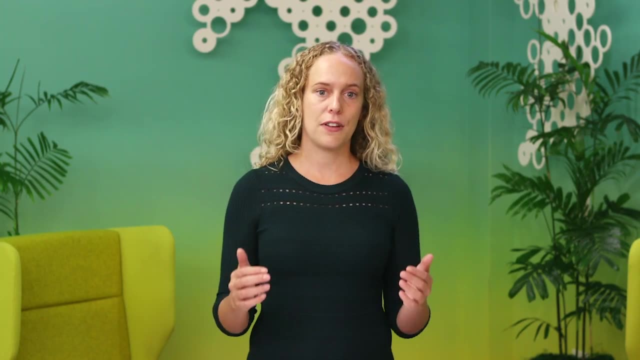 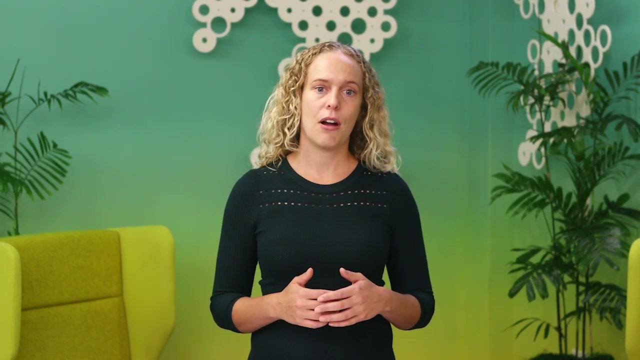 in the project goals. You need to be aware of scope risks, because the deliverables of your project might not be acceptable to your stakeholders or customers and that may defeat the purpose of the entire project. While time, budget and scope risks are very common, there are other types of external risks. 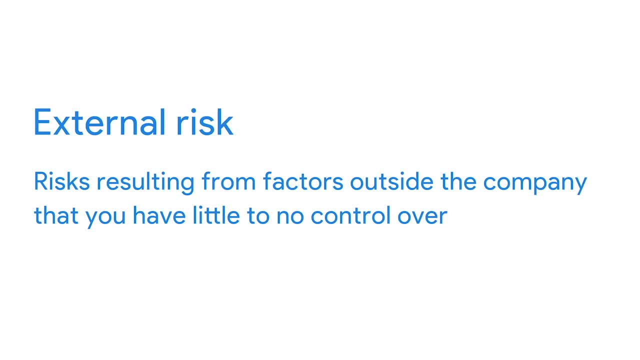 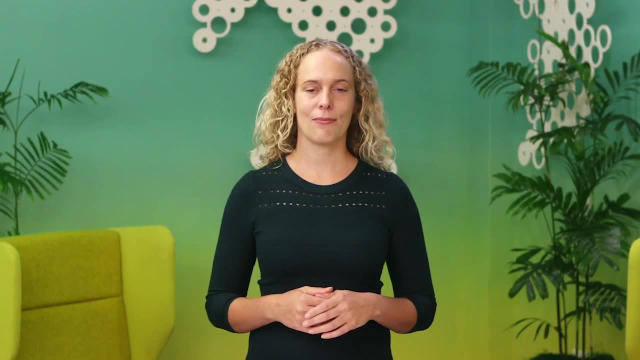 that you should be aware of. By external risks, we're referring to risks that result from factors outside of the company that you have little to no control over. For example, your project could be impacted by an environmental risk like a major storm. 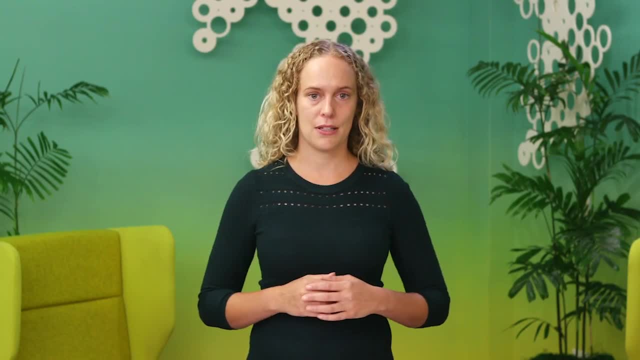 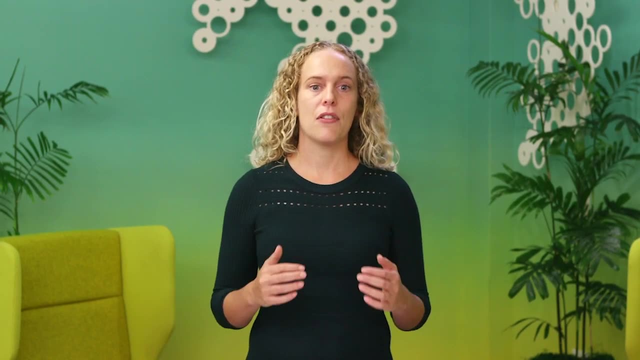 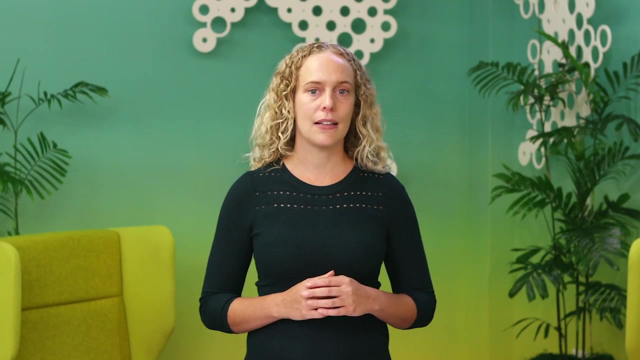 or a legal risk, like a change in regulatory requirements, And it's also important to know that there are endless types of risks. There will never be a prescription for how to identify and manage every single possible risk, But if you have a plan, you'll be better set up. 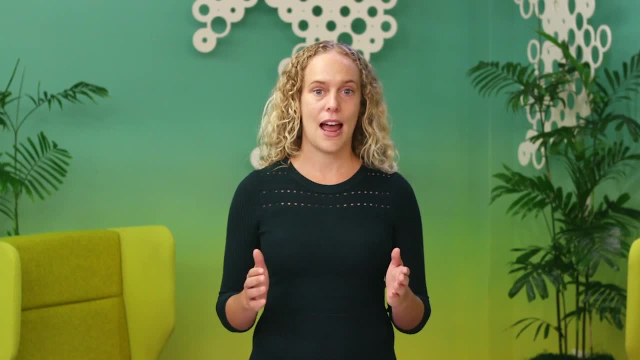 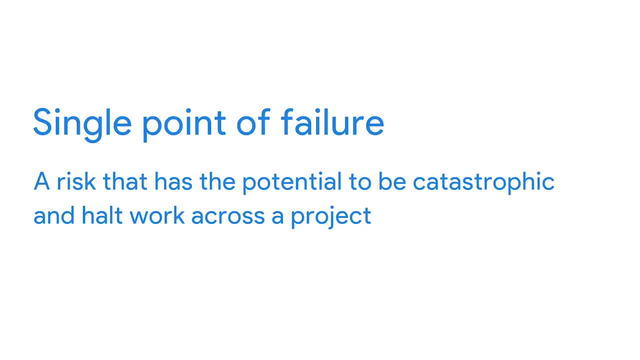 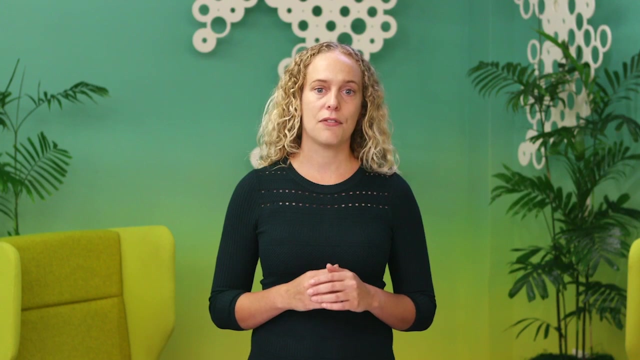 to deal with whatever comes your way. Okay, now let's discuss a certain type of risk known as a single point of failure. A single point of failure is a risk that has the potential to be catastrophic and halt work across a project. These are risks that have the power to stop an entire team. 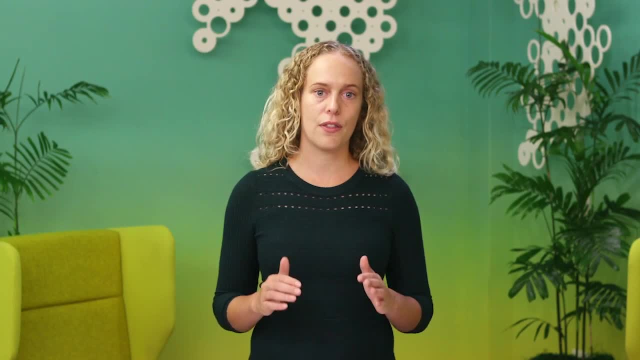 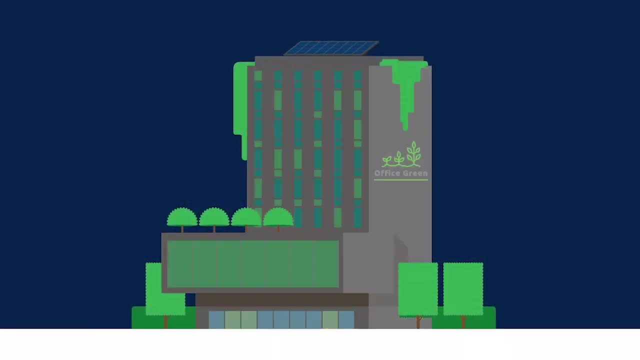 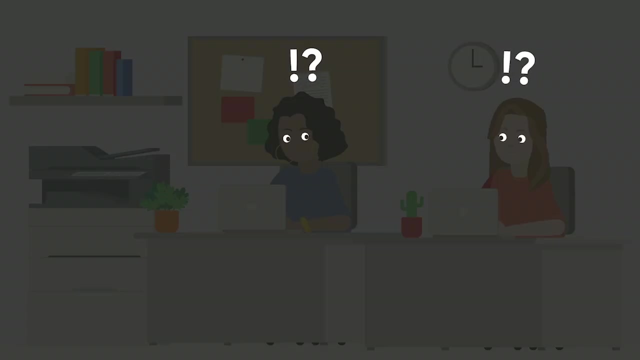 in its tracks, meaning that no one can make progress on their tasks until the issue is resolved. For example, in our office green scenario, a single point of failure might be a power outage that takes down the internal database where every piece of information about the project is stored. Until the database is back up and running, your team won't have access to any of the information they need to do their jobs. As a result, your team won't be able to complete any of their assigned tasks. To mitigate this risk, you might budget. 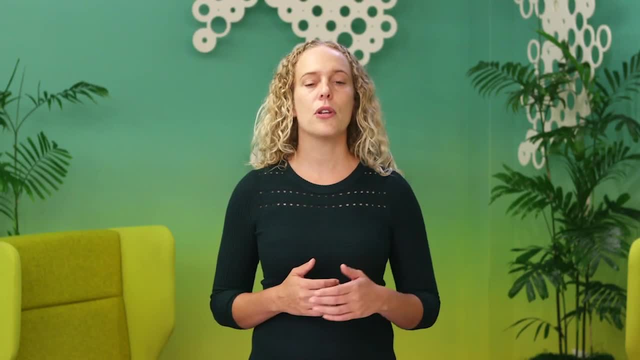 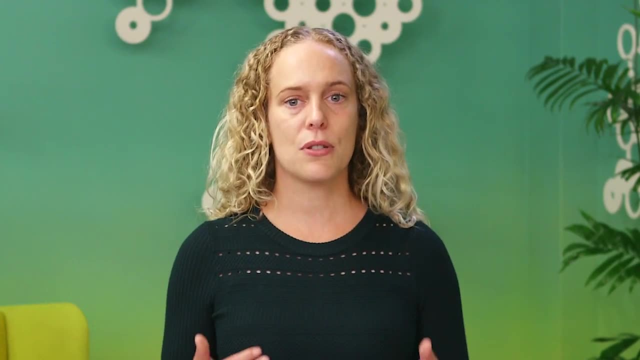 for a separate cloud service to serve as your backup for all of your project documentation and information. As the project manager, you'll need to identify and monitor potential single points of failure in your project, since they can be detrimental to the project timeline, budget and scope. 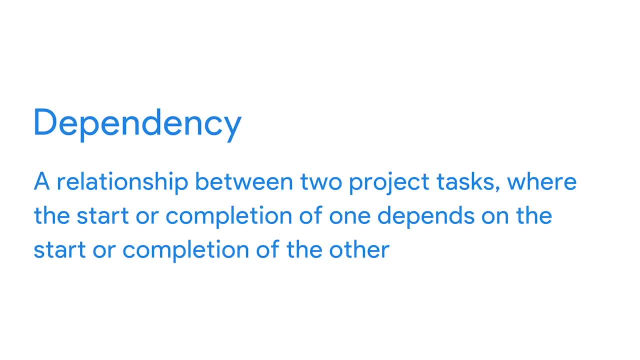 Another source of risk to be aware of are dependencies. A dependency is a relationship between two project tasks. A dependency is a relationship between two project tasks. A dependency is a relationship between two project tasks Where the start or completion of one depends on the start. 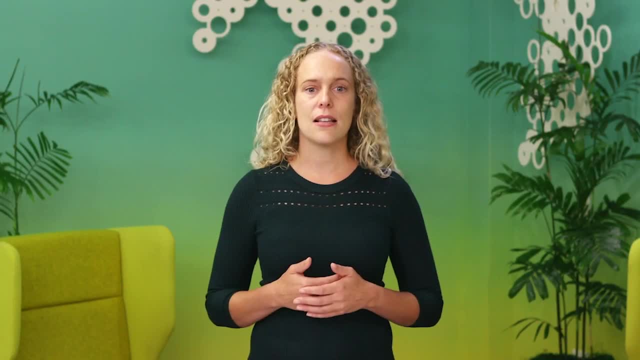 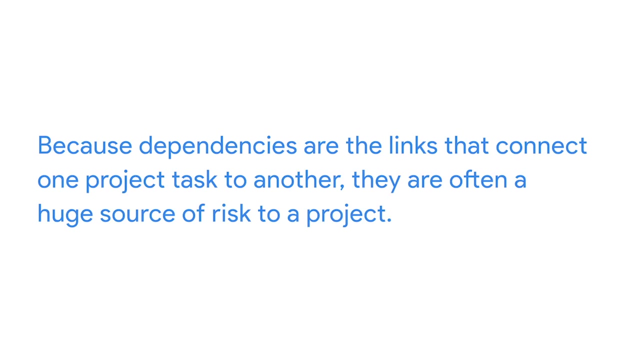 or completion of the other. In other words, dependencies are like links that connect one project task to another. A dependency must be addressed before the task can be completed or before another task can begin, Because dependencies are the links that connect one project task to another. they are often a huge source of risk to a project. For example, imagine that you've tasked a teammate with hiring a local plant supplier. Until they've signed a contract with the supplier, your team can't place any orders. That's a dependency. 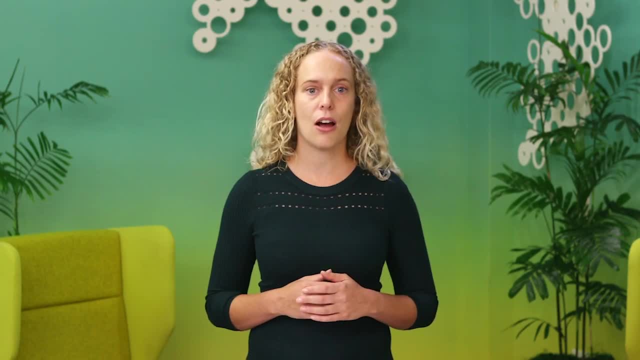 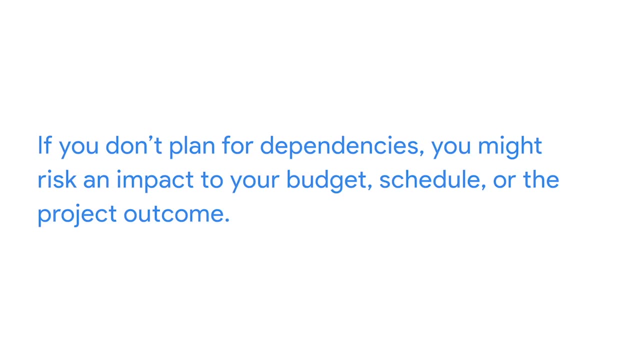 Now here's where the risk comes in. If your teammate doesn't meet the hiring deadline and then goes on vacation for a week, this could delay your project timeline. Not great right? If you don't plan for dependencies, you might risk an impact to your budget. 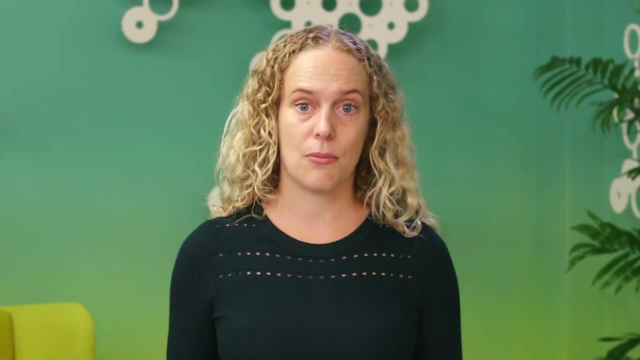 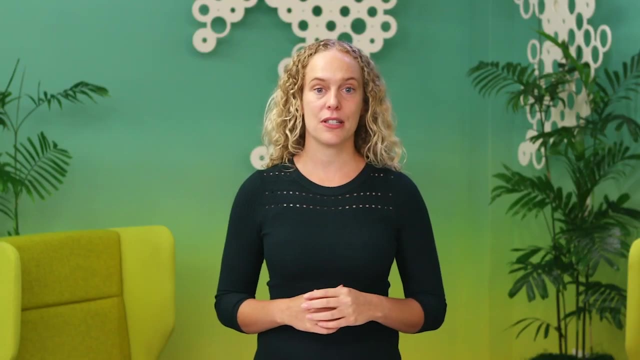 schedule or project outcome. To prevent something like this from happening, you might ask a teammate to share their out-of-office plans with you at the start of the project. This helps you to stay aware of everyone's schedules, ensuring that there are backup plans in place. 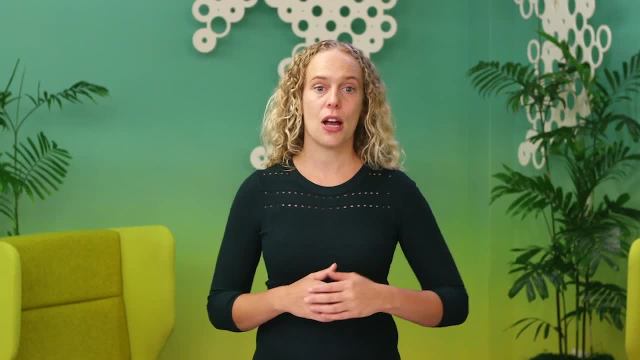 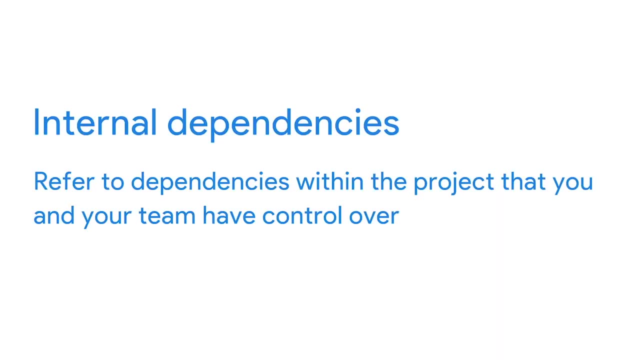 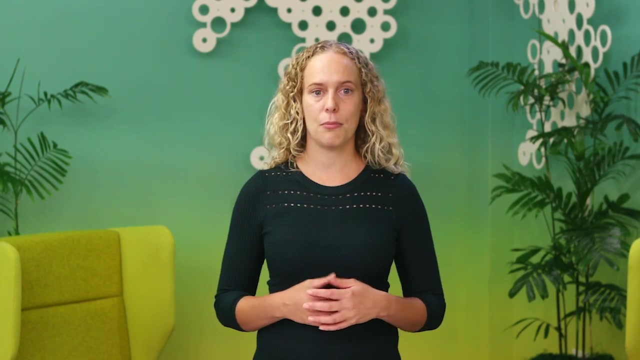 to maintain your project schedule. There are two types of dependencies: internal and external. Internal dependencies refer to dependencies within the project that you and your team have control over. For example, you'll need to secure approval on a website design before development can begin. 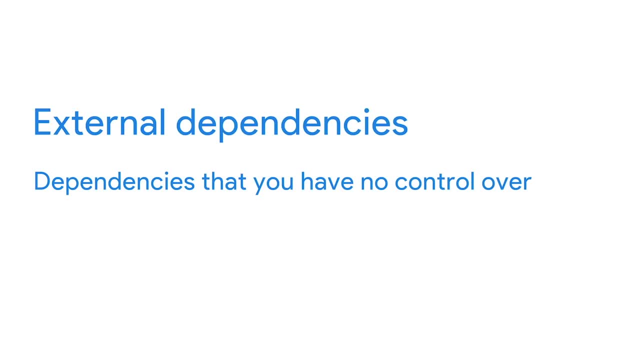 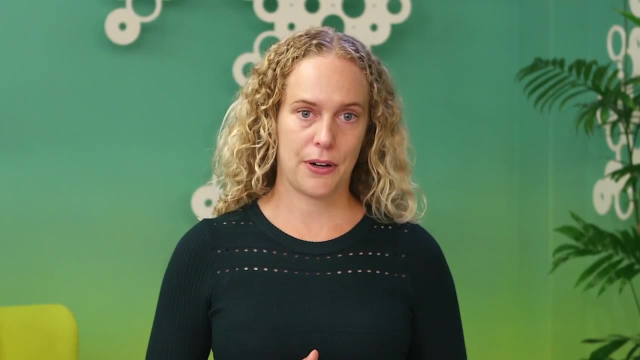 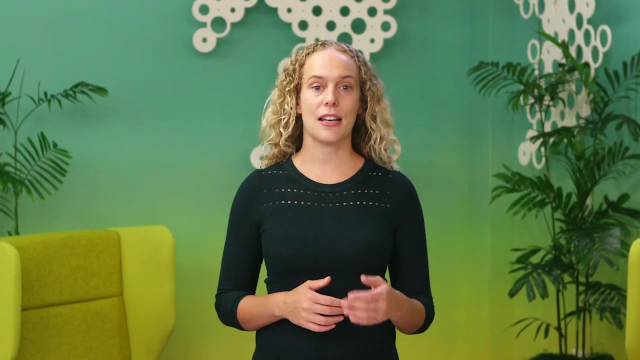 On the other hand, external dependencies are dependencies that you have no control over. For example, the farm that your plant vendor works at might have experienced a lighter rain season this year, meaning that they'll have fewer plants to sell. There are many different risks that can impact your project. 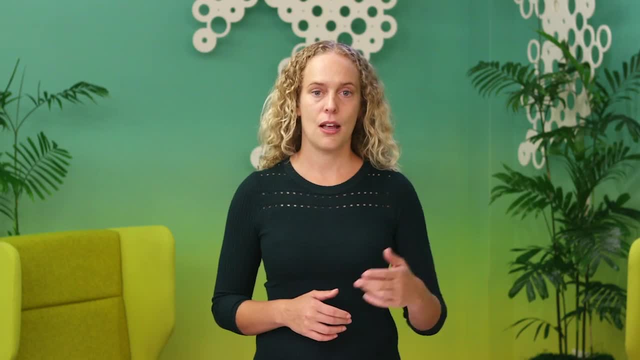 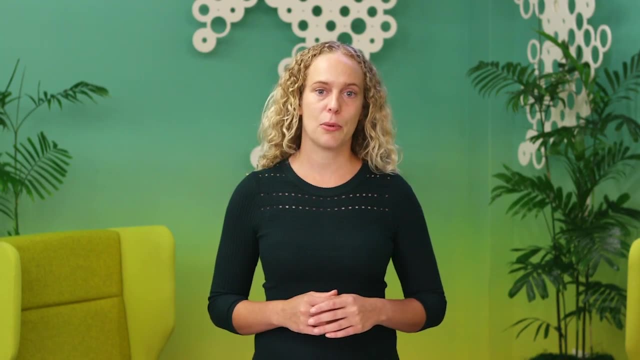 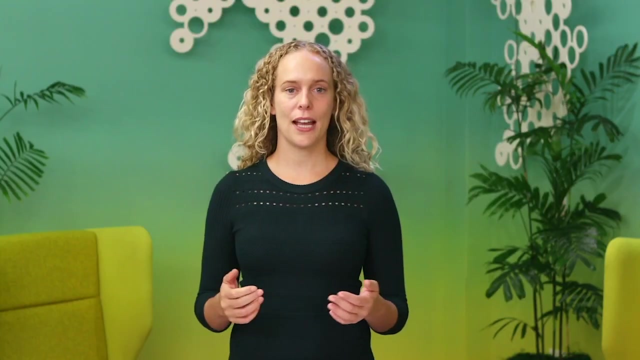 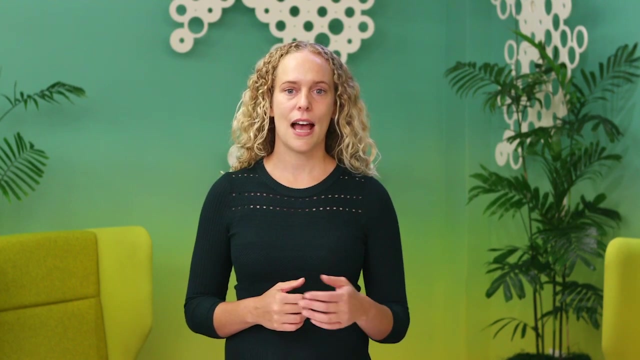 from time risks to budget risks to scope risks. But remember, no project is risk-free And with careful upfront planning, you can do your best to prevent risks from occurring. Okay, so you've learned how to identify your project's risks and assess them using a probability and impact matrix. 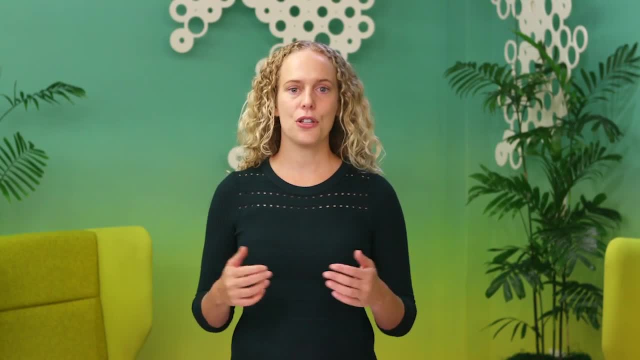 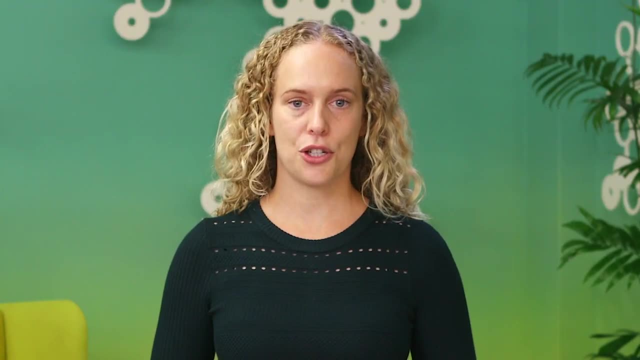 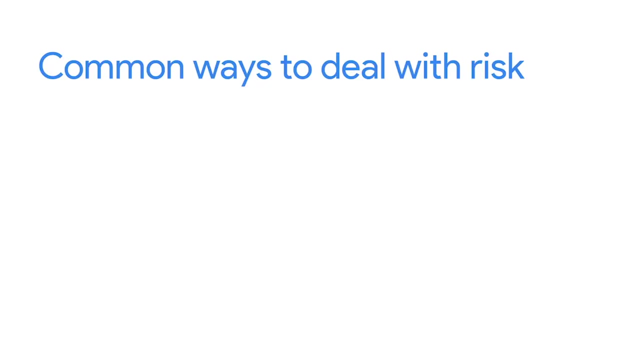 Now that you know which risks require your attention, how do you determine what to do about them? This is where risk mitigation planning comes in. Risk mitigation planning is about finding ways to eliminate or reduce the impact of potential risks to your project. There are four common ways to mitigate risk. 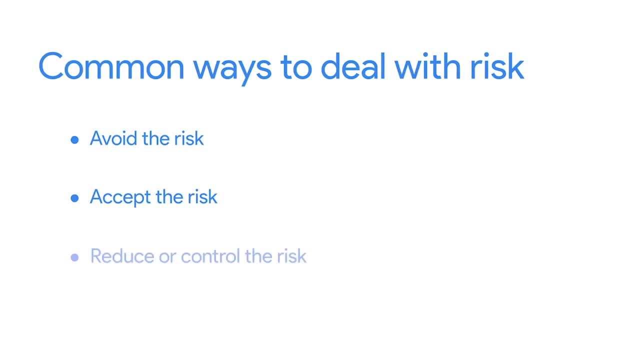 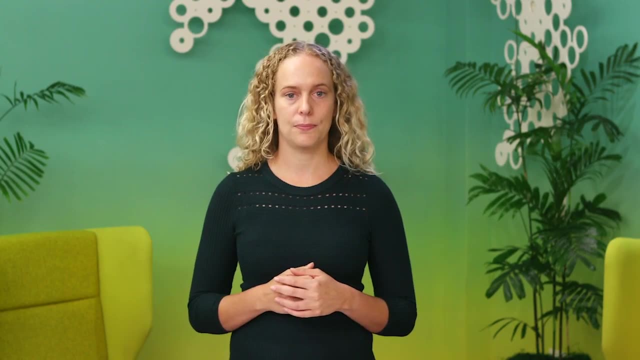 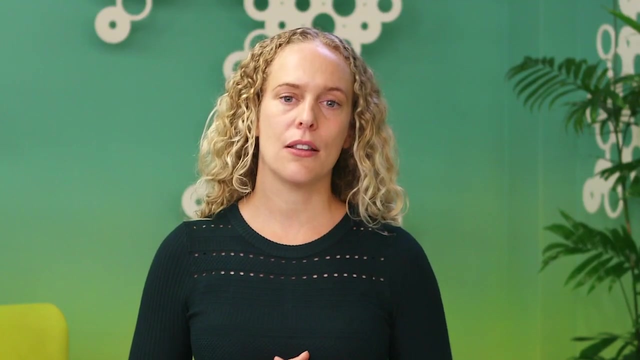 You can avoid it, accept it, reduce or control it or transfer it. Let's discuss each option using the office green example. Sometimes you can avoid the risk altogether, For example, if you learn that a certain contractor you've considered working with on your office green project. 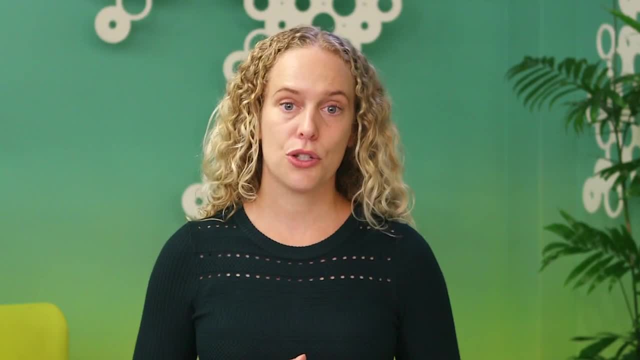 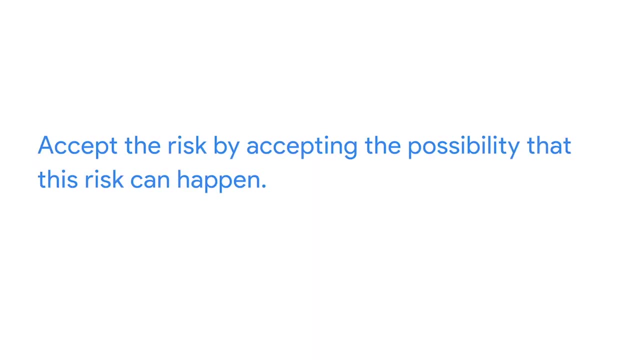 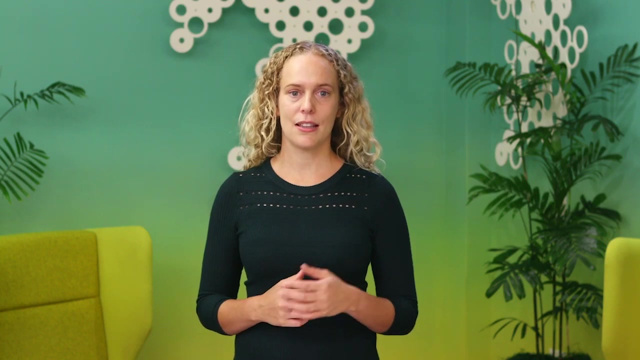 has a poor reputation for meeting deadlines, then you might choose to avoid that risk by hiring a different contractor. You can also accept the risk, especially ones that you deem low in probability and impact. In this case, you're accepting the possibility that this risk can happen. 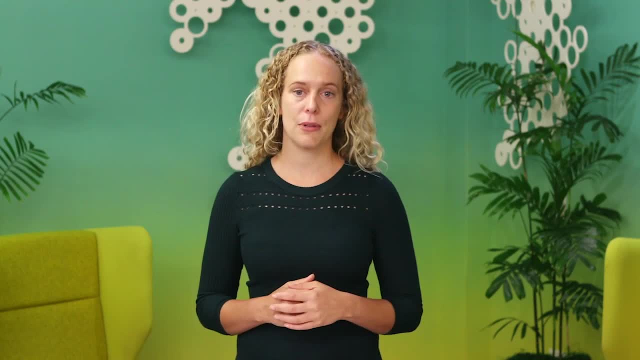 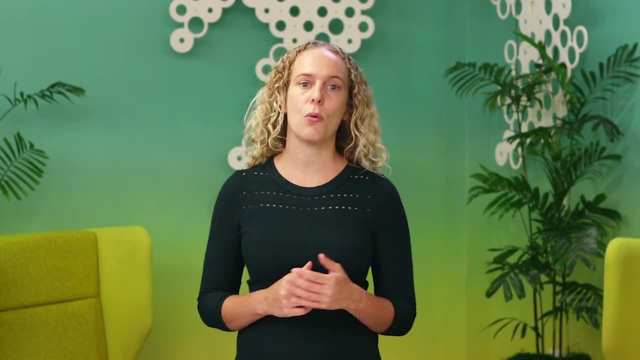 You've agreed to monitor it throughout the project and you'll ultimately be okay with the risk if it does happen. For instance, maybe your plant supplier tells you that one of the planter styles you've requested is backordered. The supplier is confident that they'll have time. 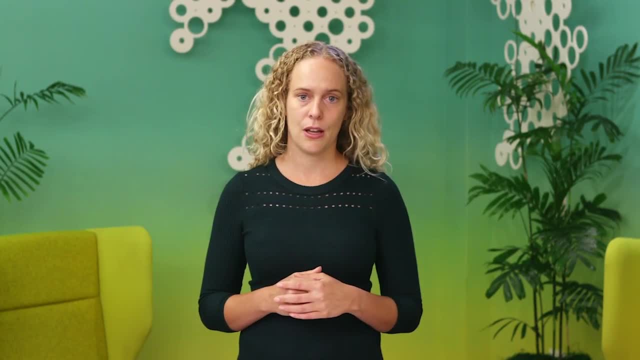 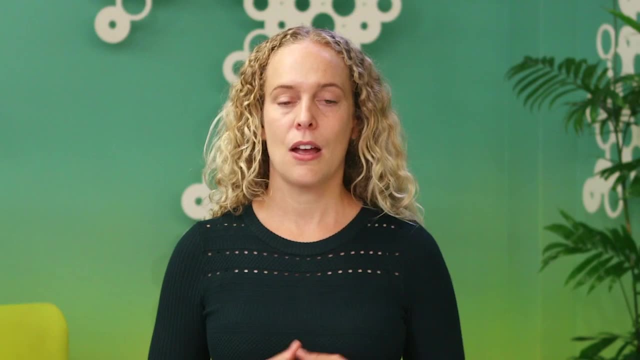 to restock the planters without delaying your project schedule, But if there is an issue with their restock shipment, this could delay deliveries to your clients by up to two days. Rather than starting over with a new supplier, you decide that it makes more sense to accept the risk. 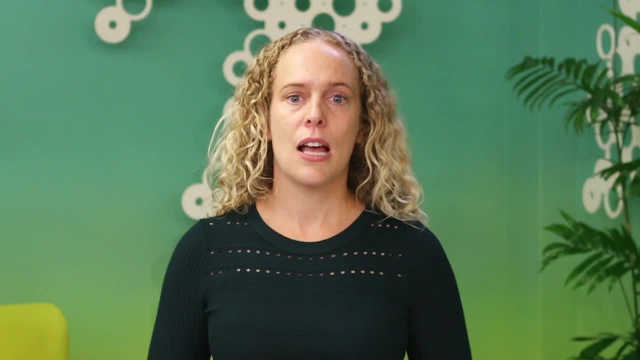 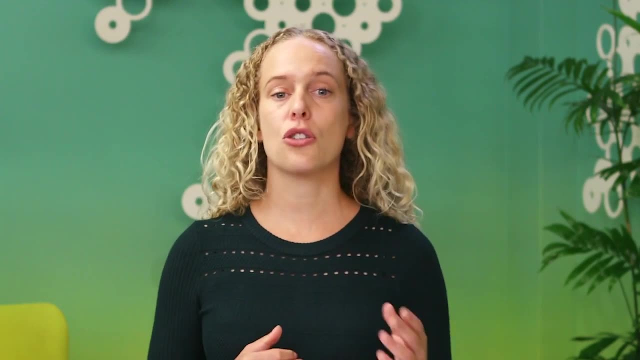 It wouldn't be ideal for this delay to occur, but you're flexible and you know that accepting this risk will save you and your team the headache of onboarding a new supplier, which could take two weeks. Another way to mitigate a risk is to reduce or control it. 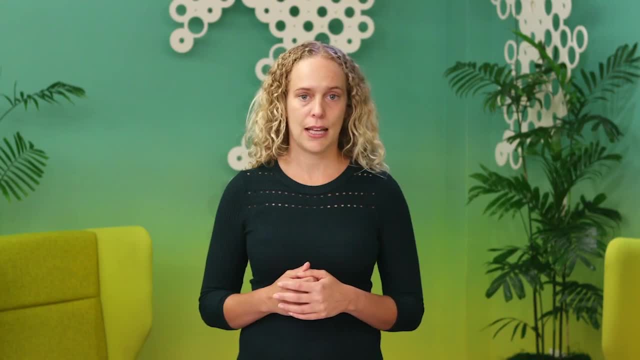 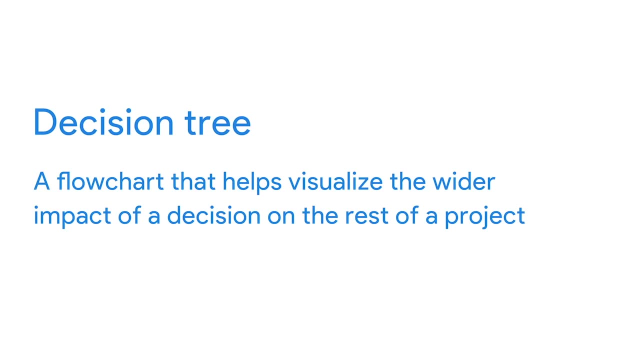 Personally, I like to use a decision tree when building mitigation plans. A decision tree is a flowchart that helps visualize the wider impact of a decision on the rest of your project. For example, you decide to hire the contractor with a reputation for missing deadlines. 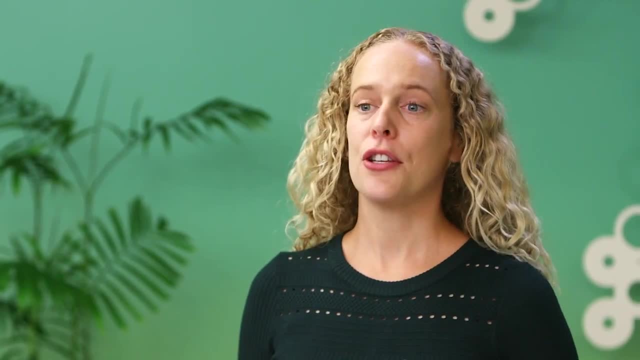 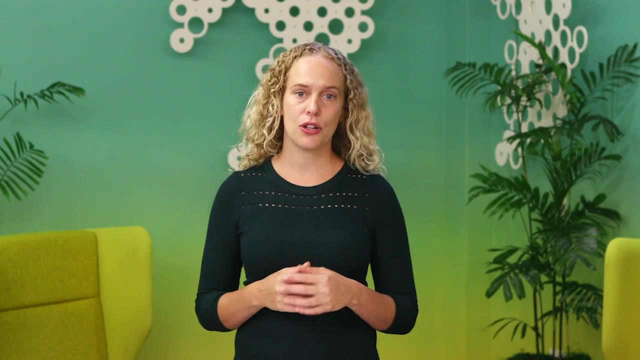 because you know they do great work. In this case, you might create a quick flowchart that visualizes the risks and potential options for addressing it, like checking in with the contractor daily, either by email or through meetings. Ultimately, you might then choose to have daily check-in meetings. 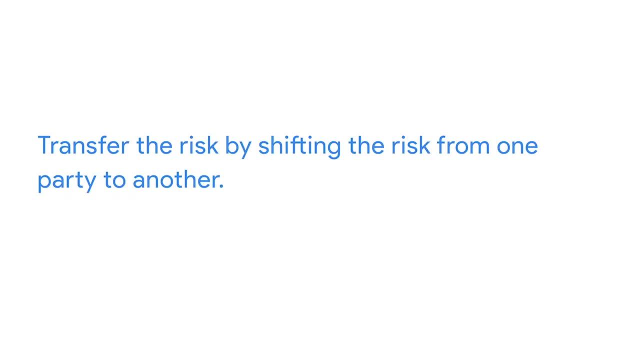 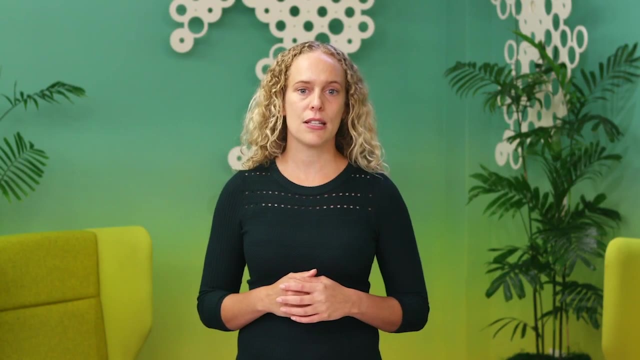 with the team to ensure that they're staying on top of their tasks. Finally, you can choose to transfer the risk. For example, you've determined that it's too risky to attempt to grow plants onsite at Office Green due to the possibility that bad weather or pests. 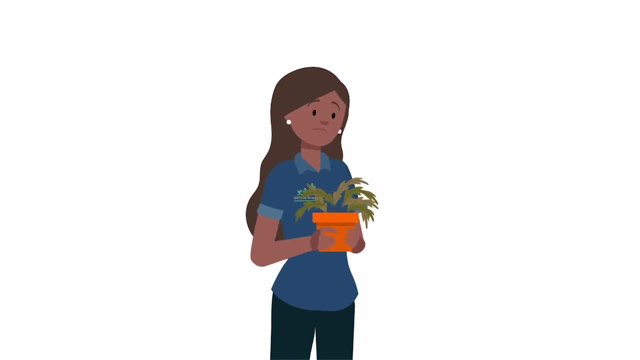 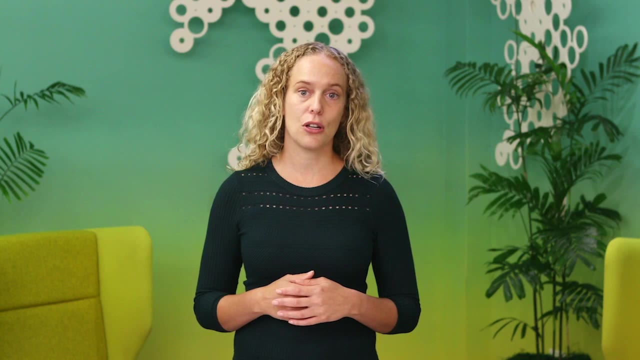 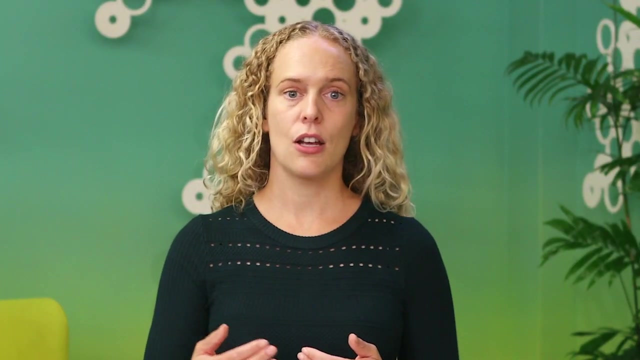 could negatively impact your product. Instead, you've made a decision to transfer the risk to another party or parties By outsourcing plant production to local suppliers. you have the power to change supplies if there's an issue with quality When you transfer the risk. you don't risk losing out on time, resources and money. So, to recap, four common ways to mitigate a risk are to avoid it, accept it, reduce or control it or transfer it. Using one of these four strategies can help you effectively take control. 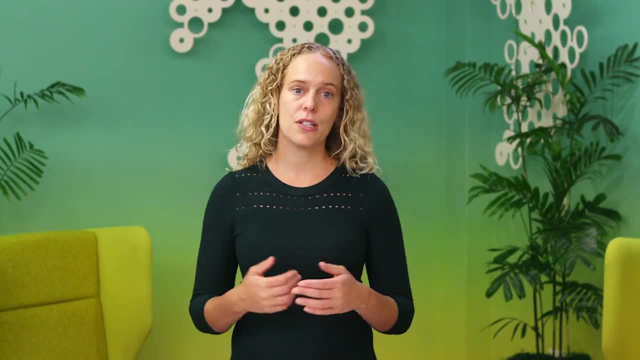 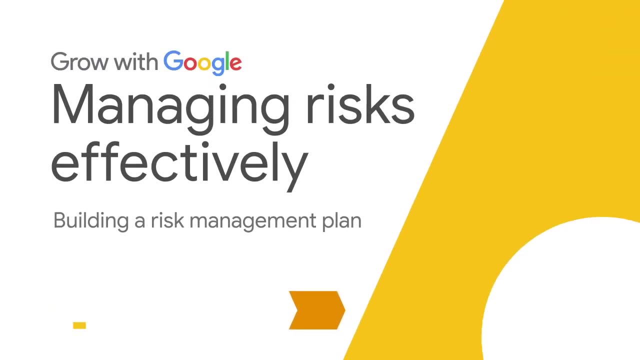 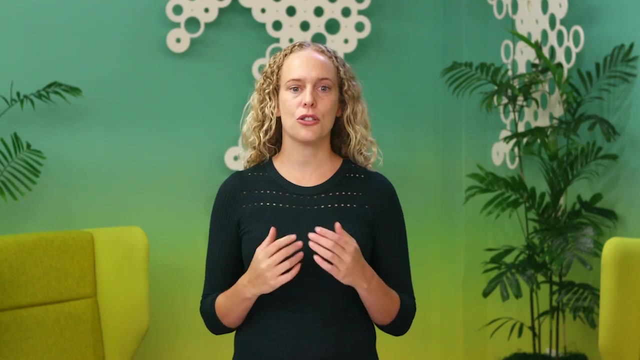 of the risks to your project Coming up, we'll discuss how to document these risks in a risk management plan. Now that you know your options for mitigating potential risks, let's discuss how to document your risk planning decisions, As you've been learning throughout this programme. 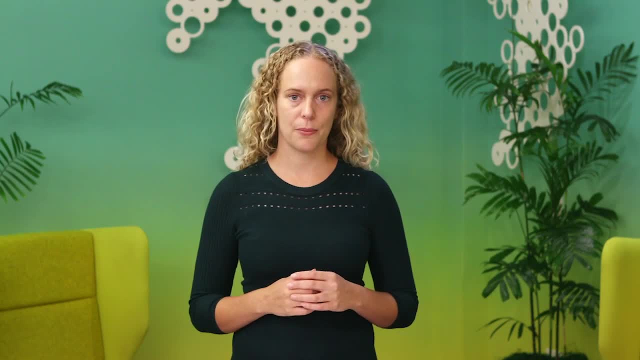 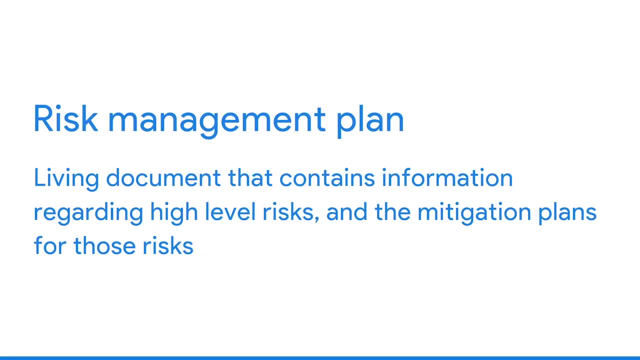 documentation is a crucial part of your role as a project manager. This is especially true when identifying risks and creating a plan to mitigate them. A risk management plan is a living document that contains information regarding high-level risks and the mitigation plan for each of those risks. 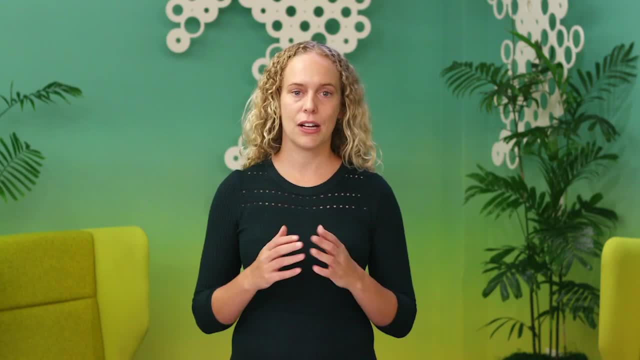 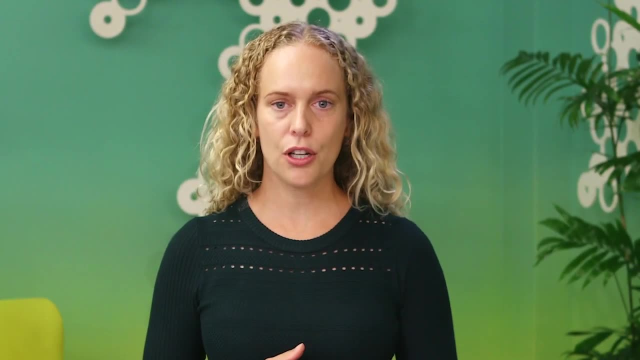 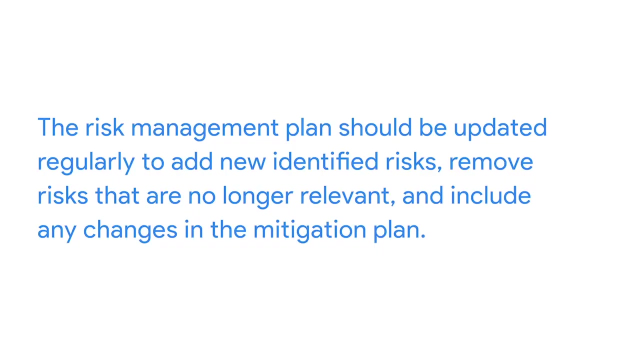 This plan helps ensure that teammates and stakeholders have a clear understanding of potential problems and a plan to address them should they occur. Risk management is an ongoing practice that you'll take part in throughout the planning and execution of a project, Since risk management evolves throughout the project. 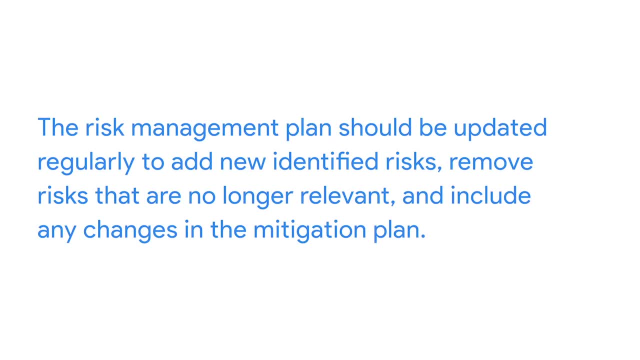 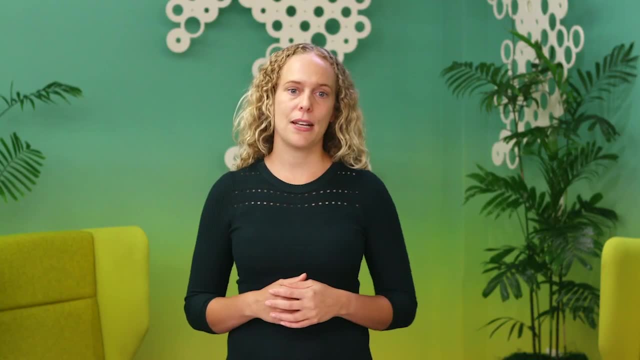 the plan should be updated regularly to add newly identified risks, remove risks that are no longer relevant and include any changes in the mitigation plans. Let's review an example of a risk management plan similar to the one we sometimes use here at Google. 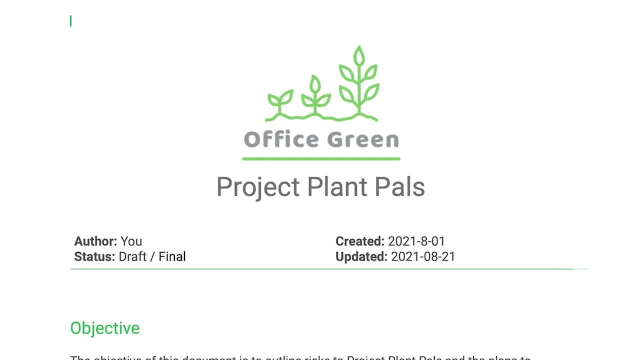 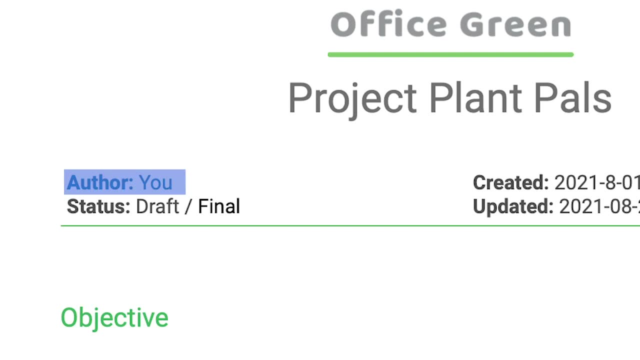 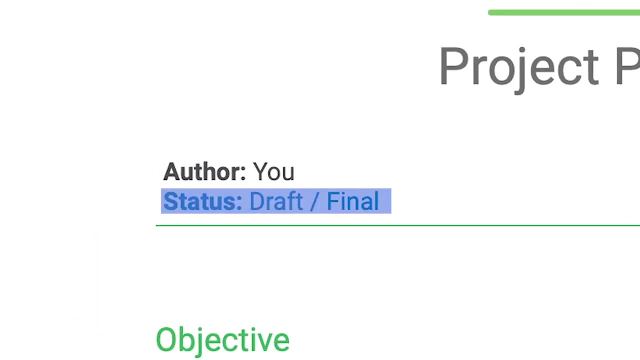 At the top of the document we include the name of the company and below it the name of the project. We also include the document author so that anyone reviewing the plan knows exactly who to reach out to if they have any questions. This template also designates a spot for the document status. 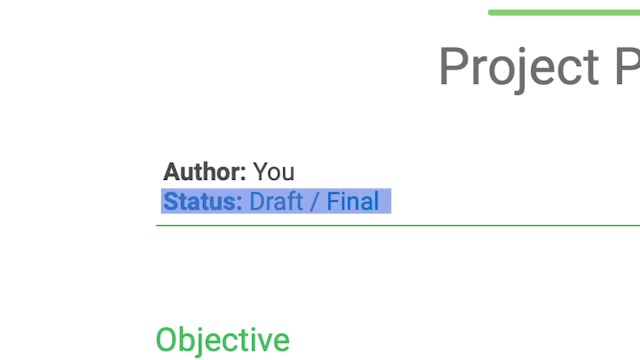 As you're building your plan, you can list the status as in progress. Once the plan is complete, you can change the status to final. We've also included helpful details like when the document was created and when it was last updated, Details that you can use to identify risk management. 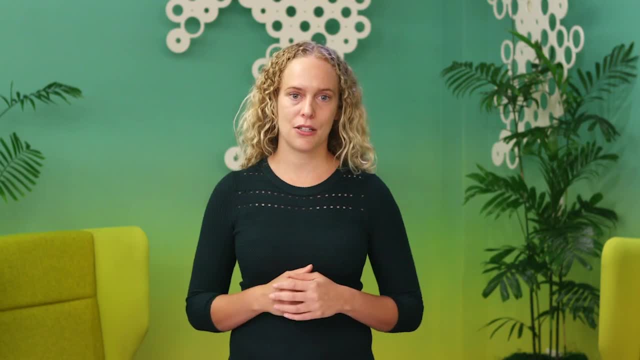 such as when the plan was created and when it was last updated, can also be used to identify risk management. Details like these might seem small, but it's best practice to include them. That's because being transparent about dates provides stakeholders with a sense of how up-to-date the document is. 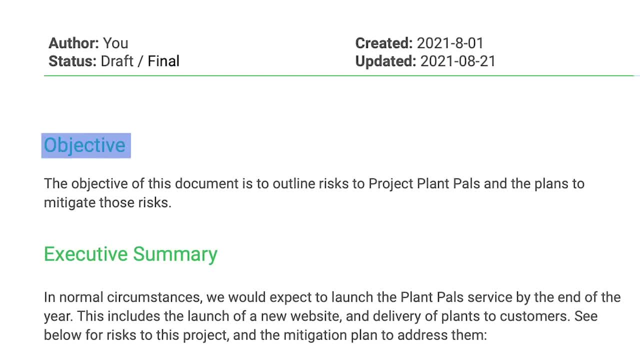 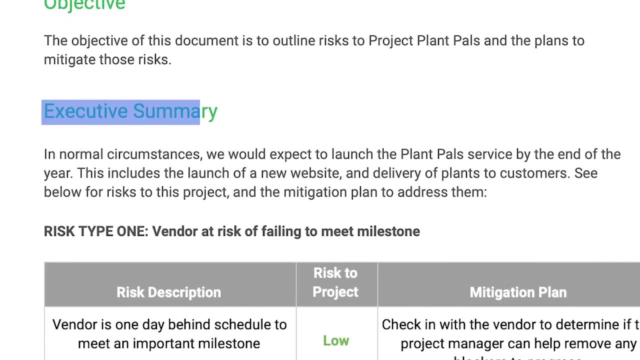 Below these details we have the document objective. Here we've written that our objective is to outline mitigation plans for project plant POWs. Below that we've added an executive summary of our project. Executive summaries should include a brief introduction to the normal conditions of a project. 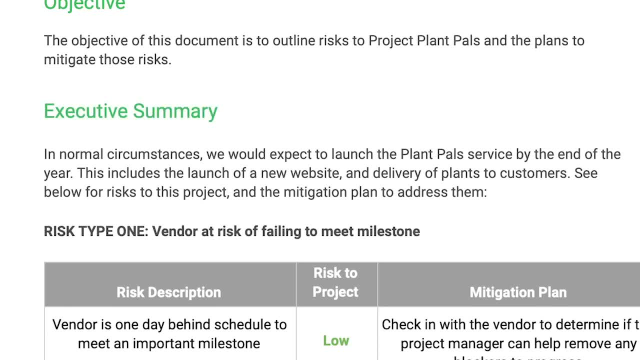 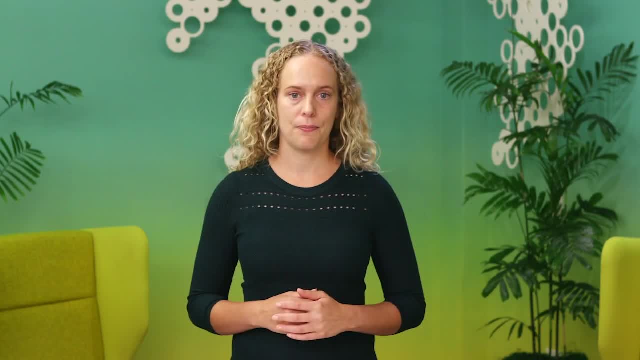 Executive summaries should include a brief introduction to the normal conditions of a project And an outline of the potential risks that could impact the project. Now onto the really important stuff: The risks and how we'll mitigate them. This document also includes the risk register you learned about earlier. 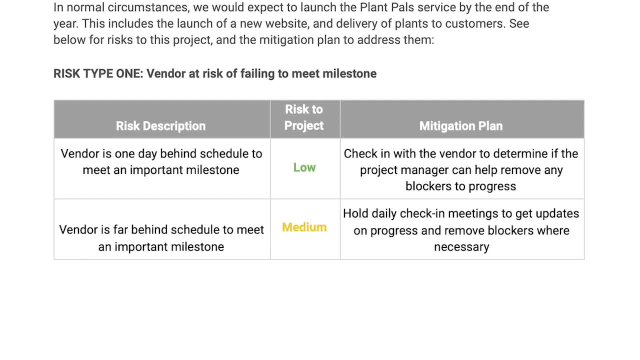 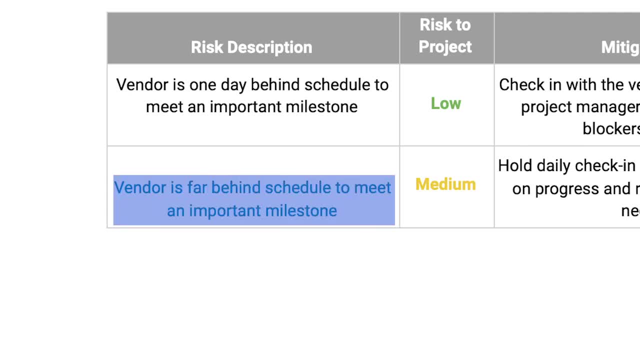 which is a table or a chart that contains your list of possible risks. Here we've outlined one of the potential risks to project plant POWs, which is the potential for the vendor to fall behind on a deadline. We've given this risk a meagre amount of time. 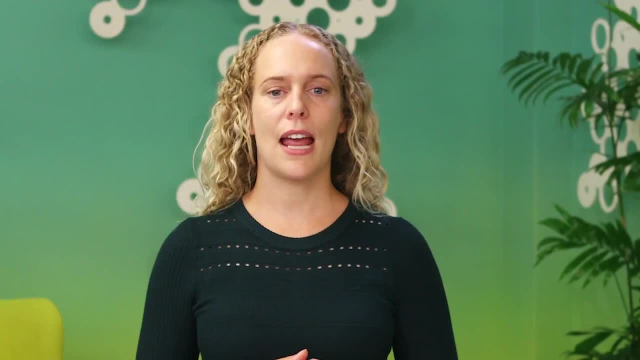 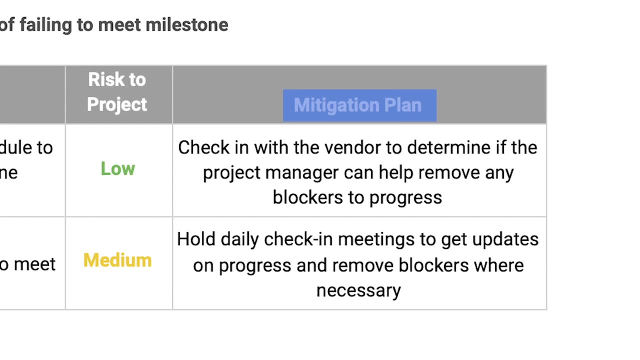 which is a medium inherent risk rating. Remember that inherent risk is the measure of a risk calculated by its probability and impact. A mitigation plan has also been included for this risk, which is to hold daily meetings with the vendor to help them stay on task. 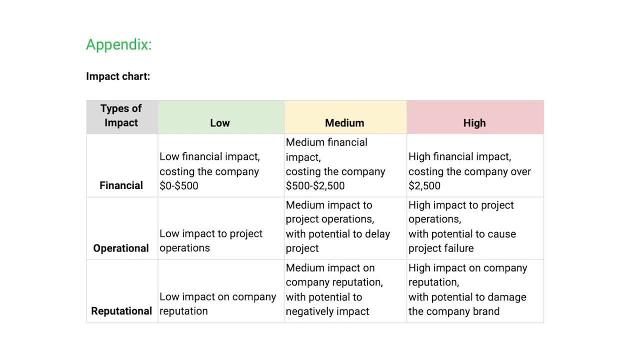 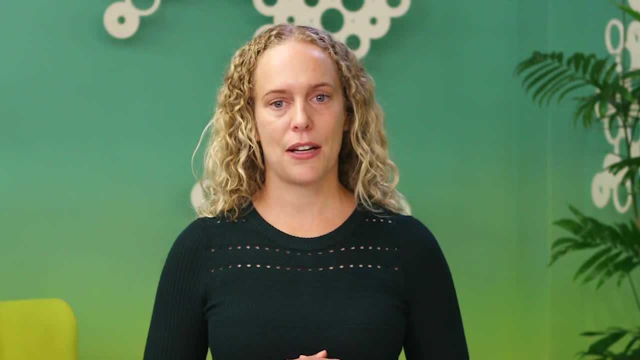 Down in the appendix of the document, you'll find the probability and impact charts, as well as the probability and impact matrix that we use to assess our risks. Once you've filled out the risk management plan, you'll share it with your team. 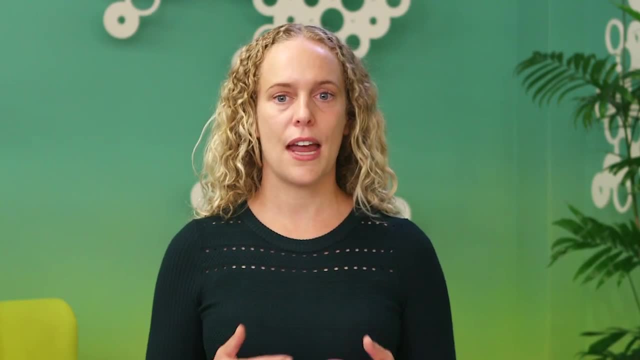 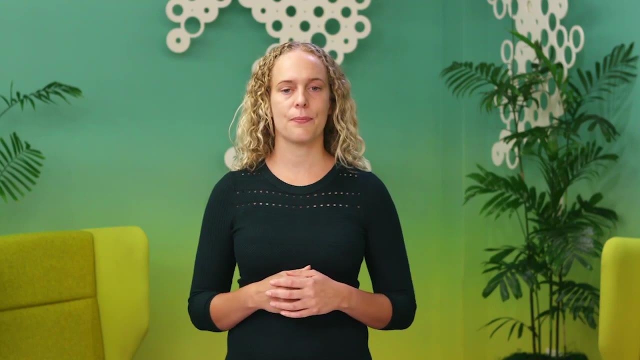 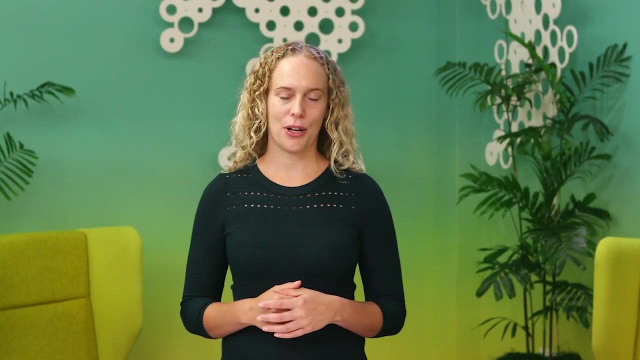 and stakeholders to get their input and to ensure that they are aligned with your plans Coming up. we'll dig deeper into the topic of communicating risks to stakeholders. See you there. As you've learned in the past few videos identifying and assessing risks, 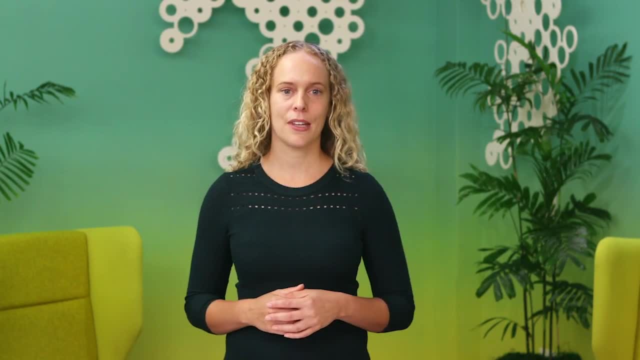 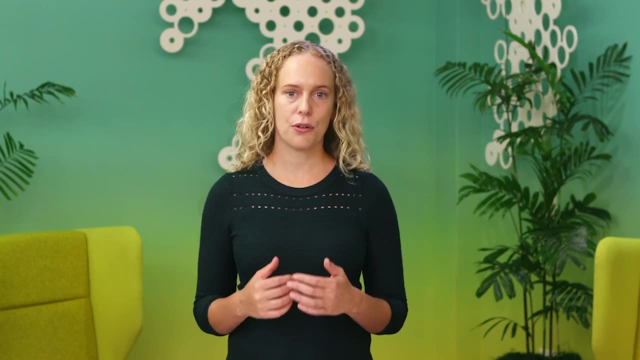 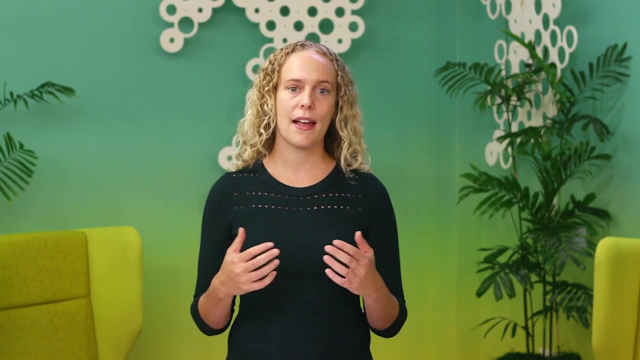 is a crucial part of the project planning process. These exercises help clarify the most important risks for you and your team and ensure that everyone agrees on which risks to plan for. But it's not enough for you and your teammates to simply be aware of the biggest risks to a project. 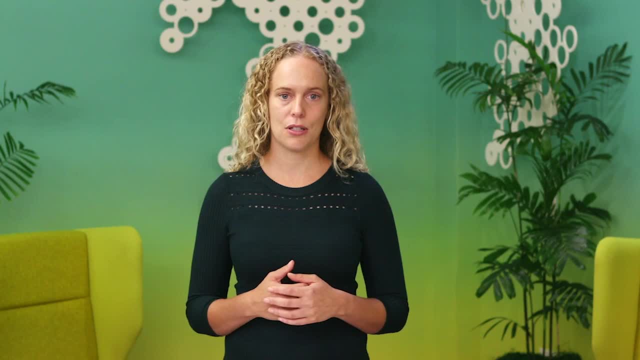 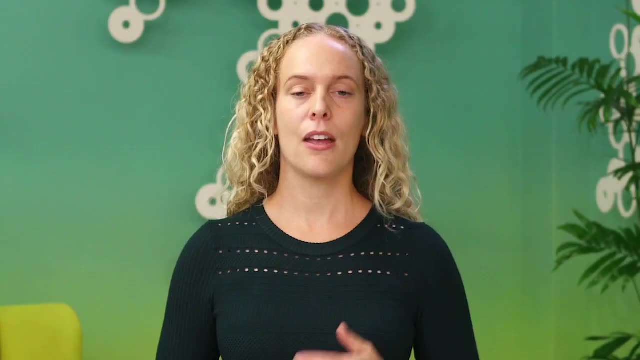 You also need to communicate these risks to your project stakeholders, whether through documentation, email, meetings or other forms of communication you've deemed appropriate. Your stakeholders need to be aware of the risks facing a project because if you don't tell your stakeholders, 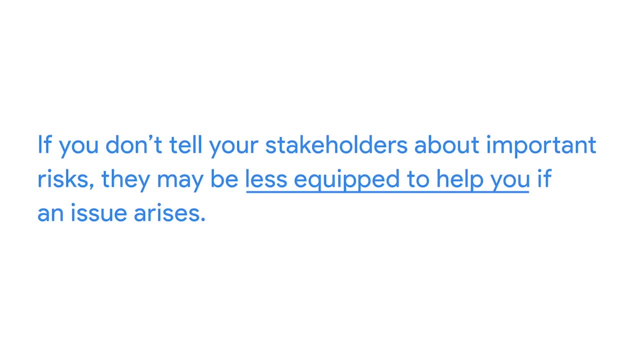 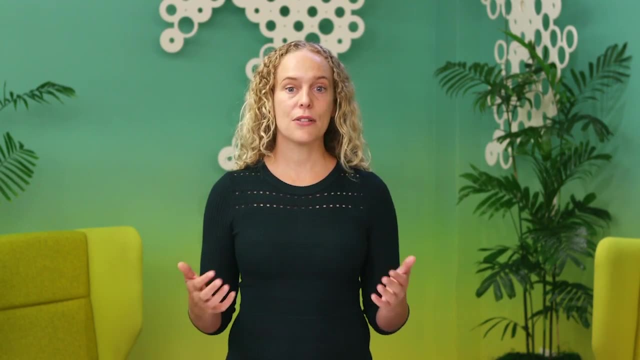 about important risks, they may be less equipped to help you if an issue does arise. For example, they might not be able to provide you with more budget, should you need it, or with more resources, should you require them. Even worse, your stakeholder might be caught off guard. 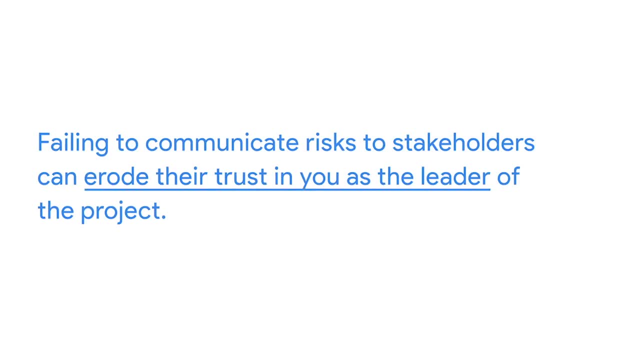 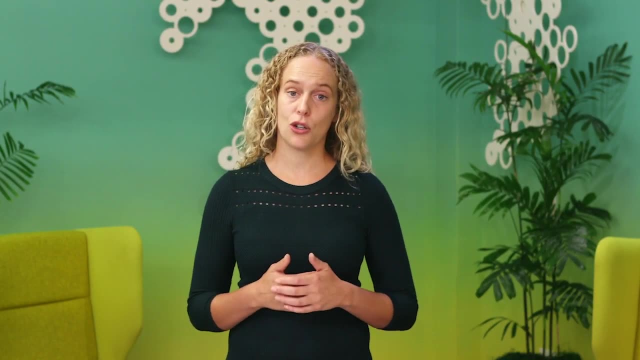 by an issue. Unpleasant surprises like these can erode their trust in you as a leader of the project. They'll likely want to know if you were aware of the possibility that this risk could occur, and they might wonder why you didn't share this information. 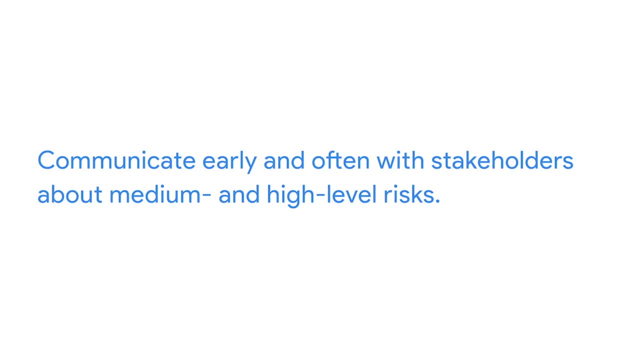 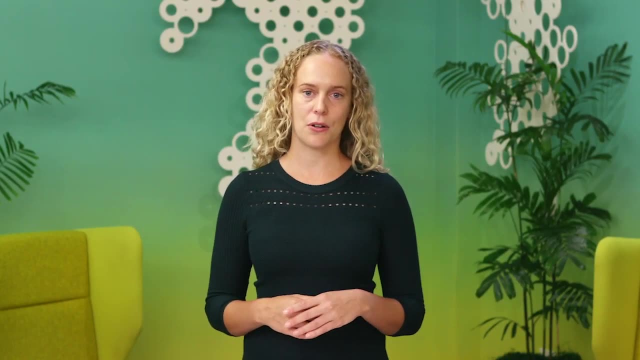 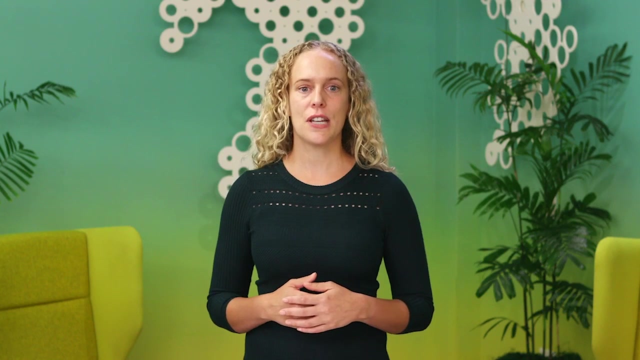 with them sooner. That's why it's important to communicate early and often with stakeholders about medium and high level risks. It sets expectations with stakeholders about what to potentially expect during the project execution phase and demonstrates that you've taken steps to mitigate and plan for those risks should they come up. 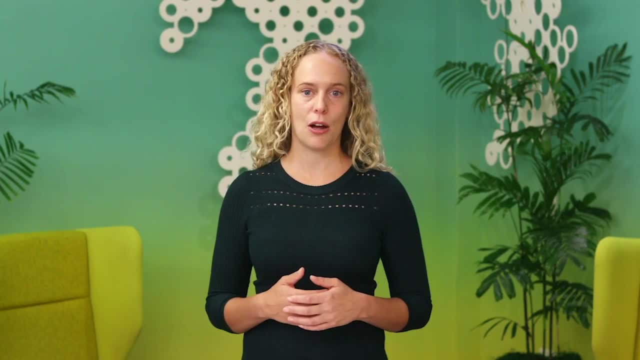 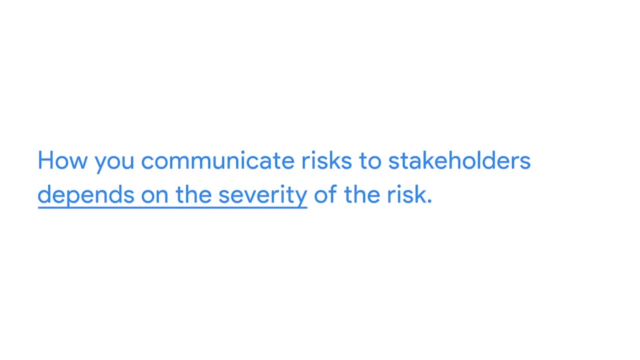 It also gives you the opportunity to suggest ways they might be able to help you if a risk does arise. So how do you communicate risks to stakeholders? How do you communicate risks to stakeholders during the planning phase? Well, that depends on the severity of the identified risk. 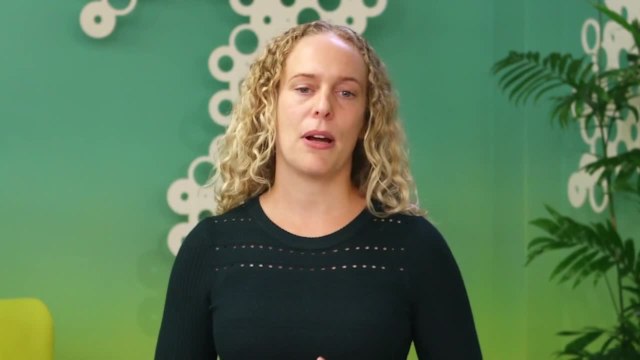 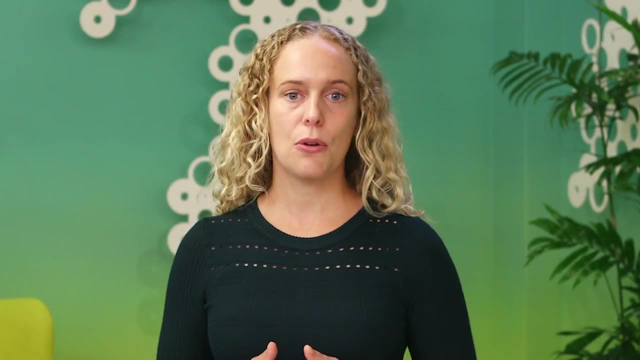 For low level risks, something as simple as an email might suffice. For example, when sending out weekly planning updates to a project stakeholder, you might list a few low level risks that are relevant to their interests and briefly explain how you'll address these risks. 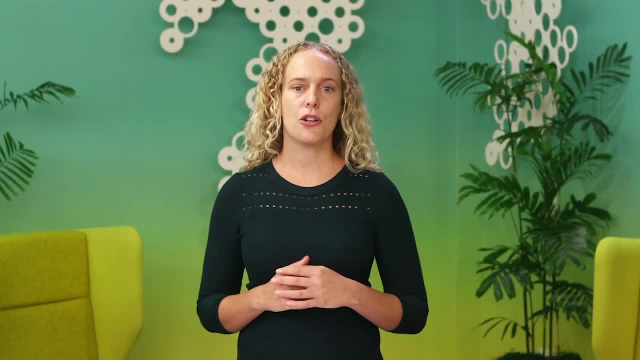 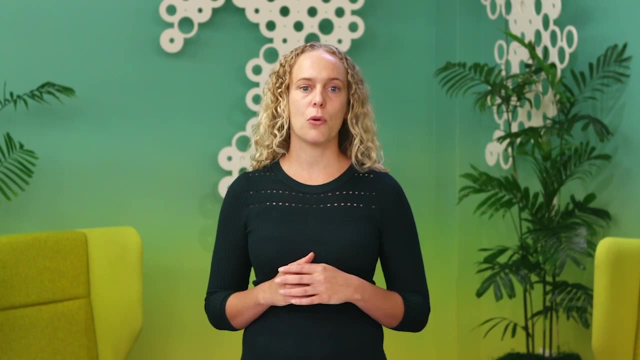 if they arise For medium level risks, you might increase your level of communication to a direct email between yourself and the stakeholder in which you outline the risk with more specifics and provide a detailed explanation of your plan to mitigate the risk. You might also link to your risk management plan. 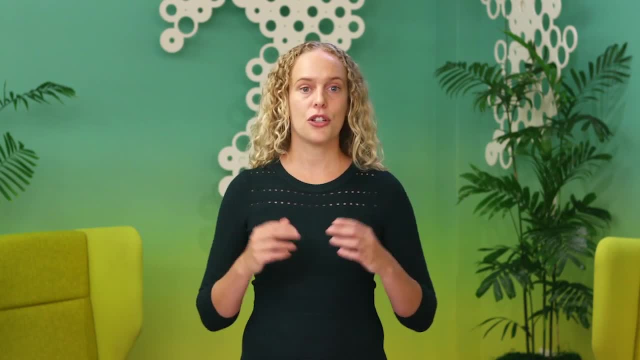 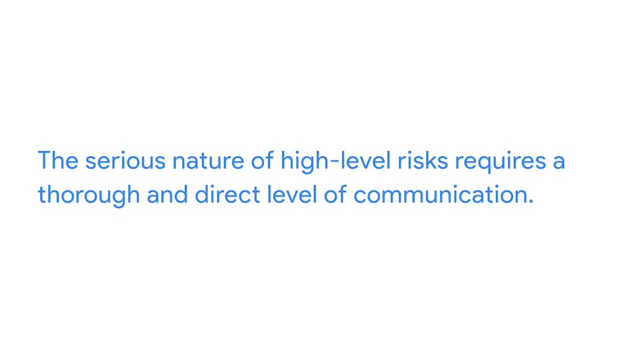 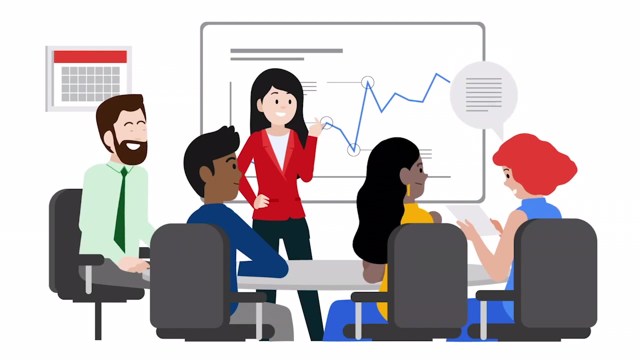 to provide them with more information and you might write urgent in the subject line to stress the email's importance. The serious nature of high level risks requires a thorough and direct level of communication When you're meeting with stakeholders to go over the project plan. 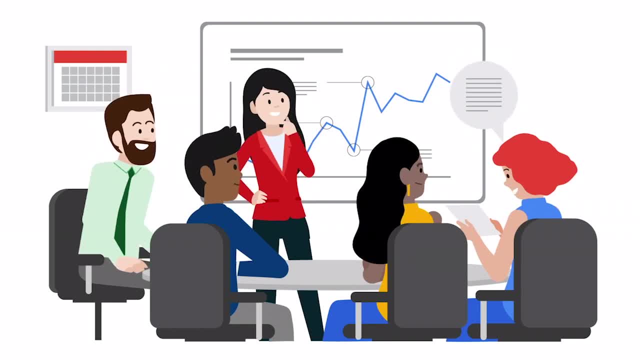 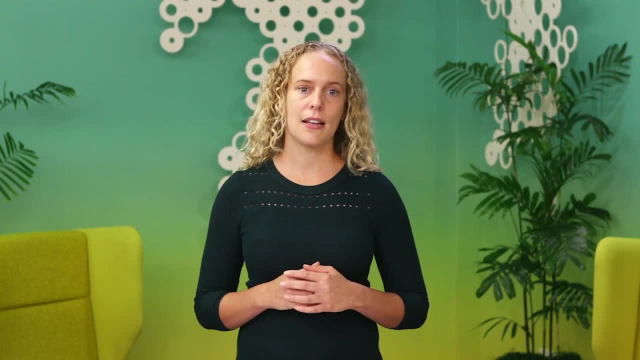 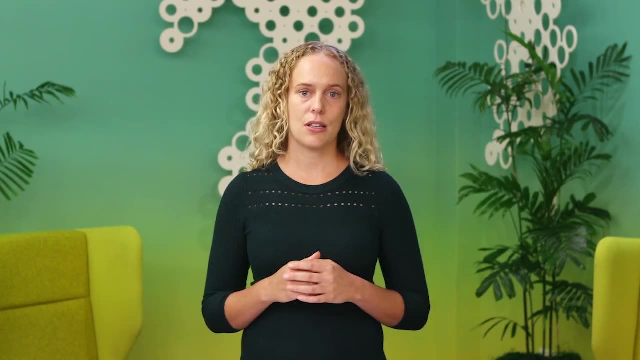 you might add an agenda item to present serious risks and your plans to mitigate these risks. You can also use this time to collect feedback on your risk management plan and ask for insights from stakeholders on how they suggest handling these high level risks. Your stakeholders might have prior experience planning. 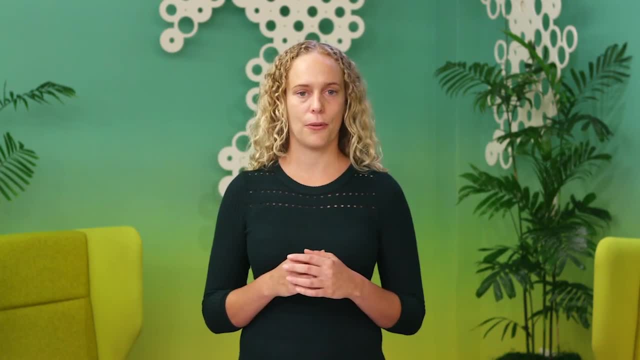 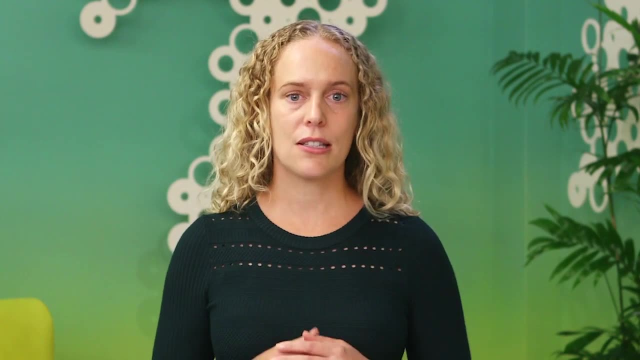 for similar risks and strategies that you hadn't considered before. Risk communication is a big part of my role here at Google As a program manager. I am constantly writing emails and delivering presentations on the status of my projects, often with the goal of sharing known risks. 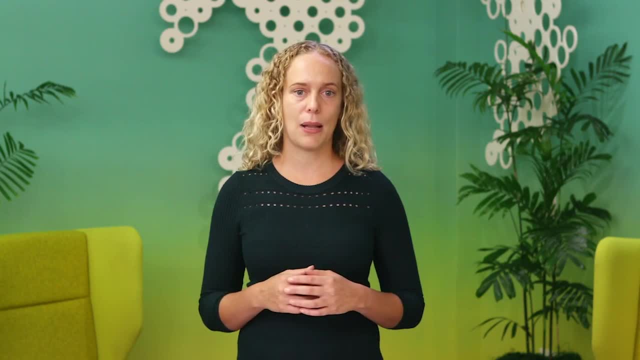 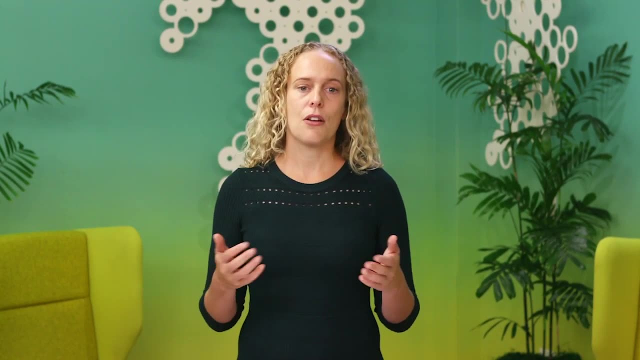 and my risk mitigation plans, And in discussing these plans with my stakeholders, we often uncover other risks that I hadn't even considered. For example, in a recent meeting I was presenting a potential new product to a stakeholder on a different team. 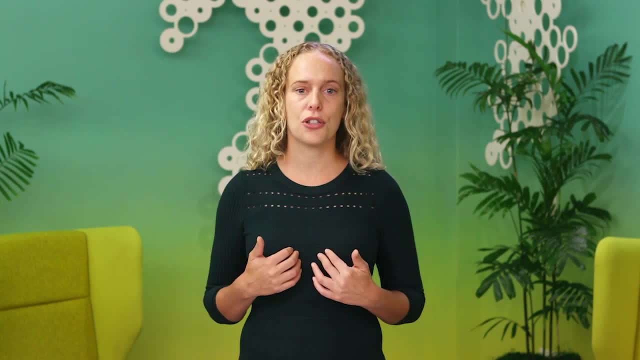 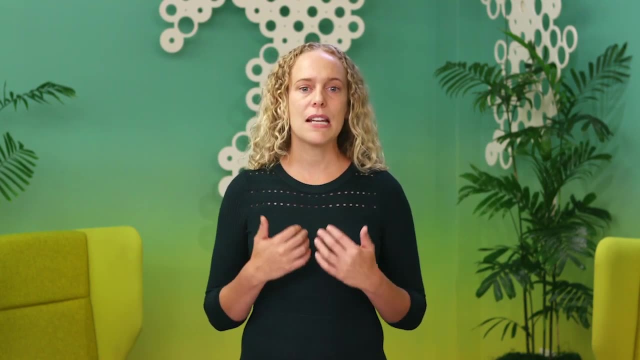 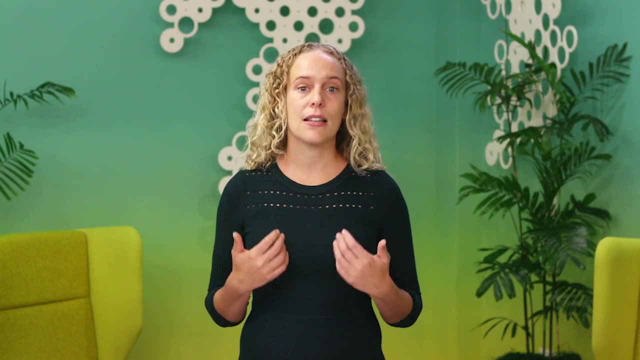 In the meeting, the stakeholder flagged their concerns that my solution might create time and resource risks that could have a negative impact on their team. This discussion gave me deeper insights of my colleagues' potential risks and of the product's users' needs, which made me realize that I needed to ask my project sponsors. 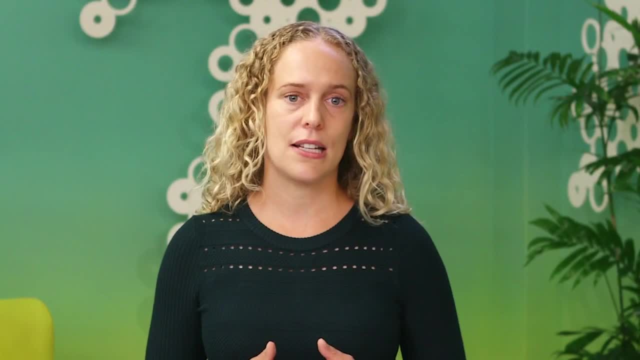 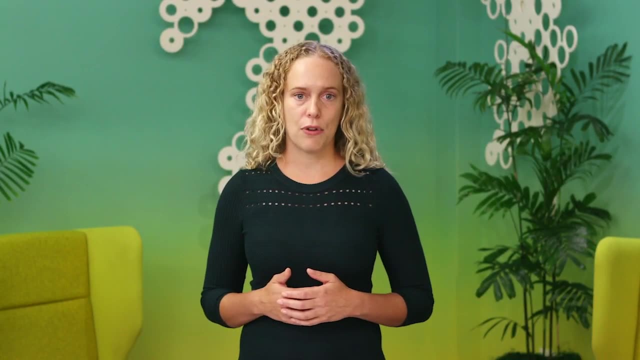 for additional budget and resources. So it's always a good idea to discuss your plans with your stakeholders. They may have a different perspective. So, to recap, it's important to communicate risks to stakeholders so that they're better able to help you should one arise, and you should tailor your 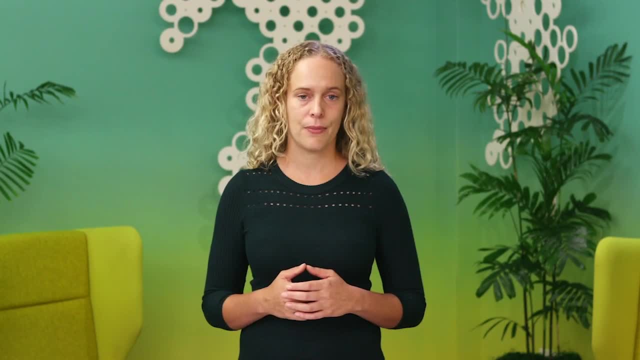 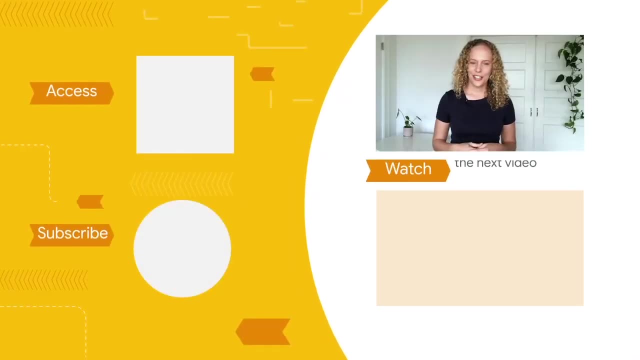 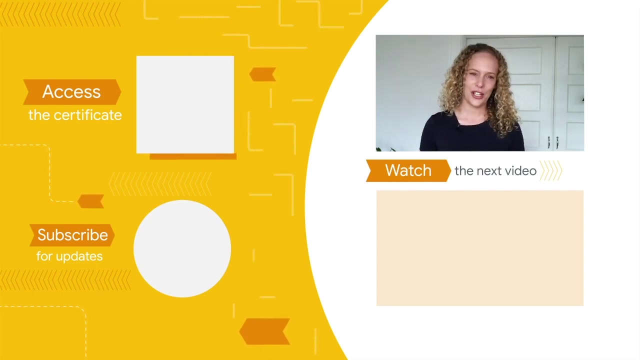 communication style according to the severity of the risk. Up next we'll review and wrap up all that we've covered. Meet me there. Congratulations on finishing this video. in the Google Project Management Certificate, Access the full learning experience, including job search help and start. 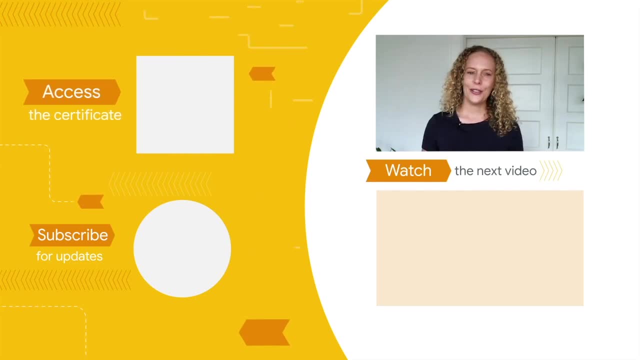 to earn your official certificate by clicking on the icon To view the next course in this video. click here And subscribe to our channel to learn more from Google Career Certificates.